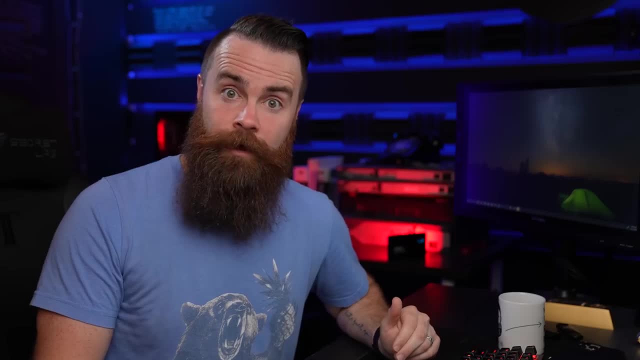 Oh my gosh. This is definitely a skill you want to add to your toolbox right now. Now, before you freak out, we're not going too deep here. You don't need to become a sequel expert unless you want to become a DBA or 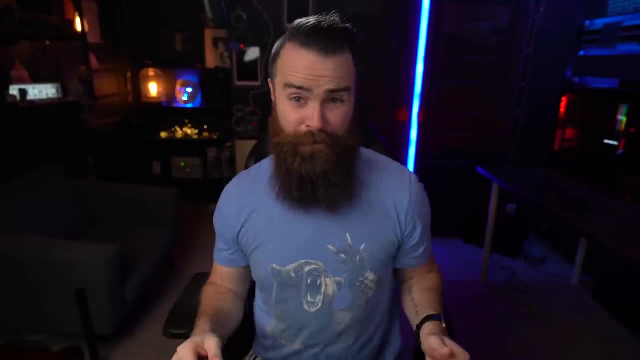 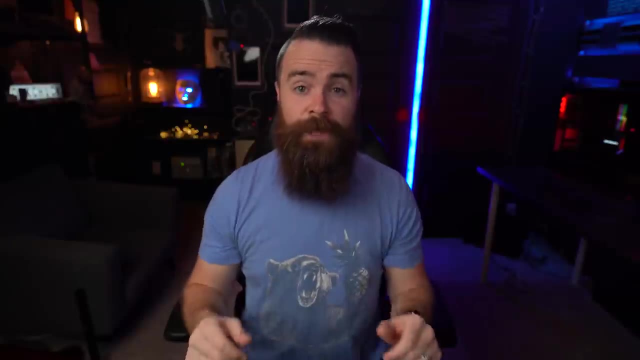 something. You poor, brave, stupid soul, but you're making bank and you're rich, but knowing the basics like, Hey, what even is a database? that goes a long way And pretty much every area of it So in this video. 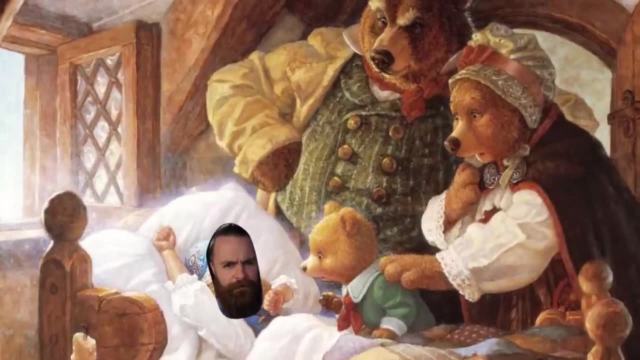 I'm going to teach you SQL, not too much like a Goldilocks amount of SQL, just enough to make you dangerous, but not too dangerous. I don't want you dropping elbows on some poor, unsuspecting tables. So by the end of this video, 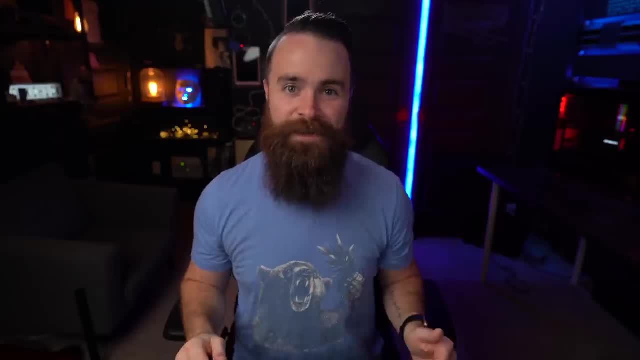 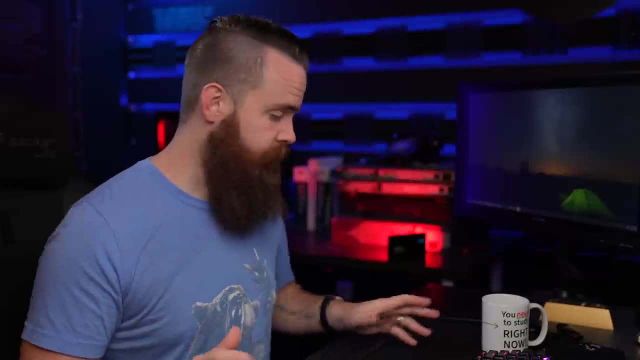 you will know how to create your own MySQL or MySQL database, And you're going to add some stuff into it: remove some stuff, query some things. So get your coffee ready. Mine is right here, And let's learn some SQL. Now, while you're sipping that coffee, getting all fueled up, 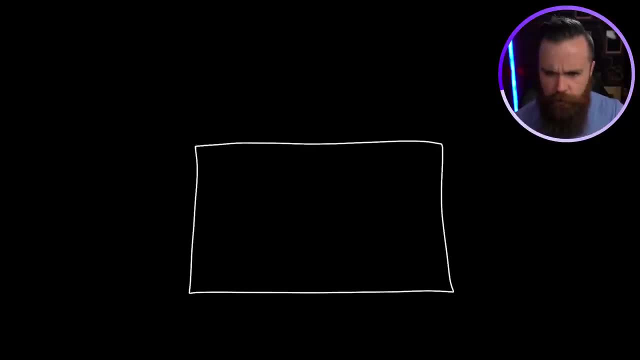 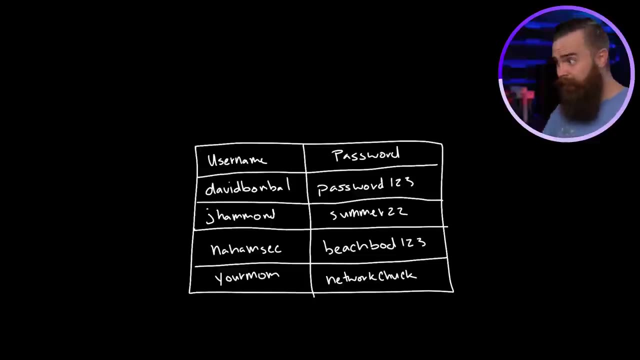 ready to go to learn some SQL? Let me tell you a scary story. Did you know that Your usernames and your passwords? they're often stored inside a SQL database And sometimes these databases spring a leak, spilling your username and password all over the dark web? David Bumble. 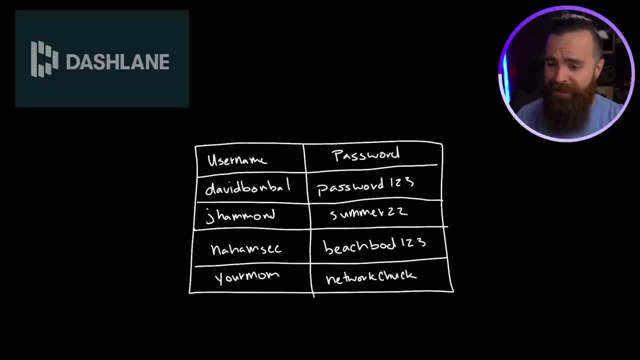 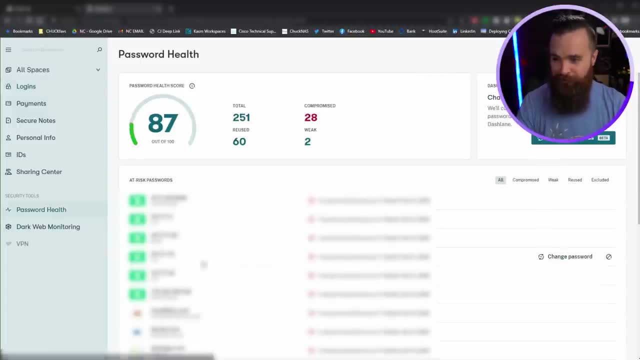 I'm disappointed. This is where our sponsor, Dashlane, comes in. Dashlane does a great job at protecting you from yourself. Come on, John Hammond. I love their password health feature, which obviously I got some work to do. I got 28 compromised passwords and two weak ones. no weakness allowed. 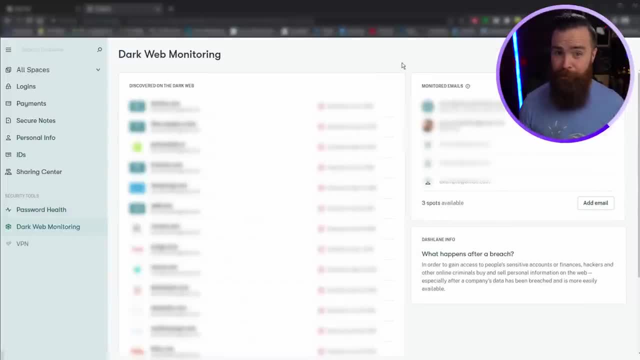 And I also love their dark web monitoring Cause- I wasn't kidding- These databases full of your passwords and emails and all kinds of stuff get hacked and leaked all the time on the dark web. They monitor that stuff for you and they'll tell you Hey. 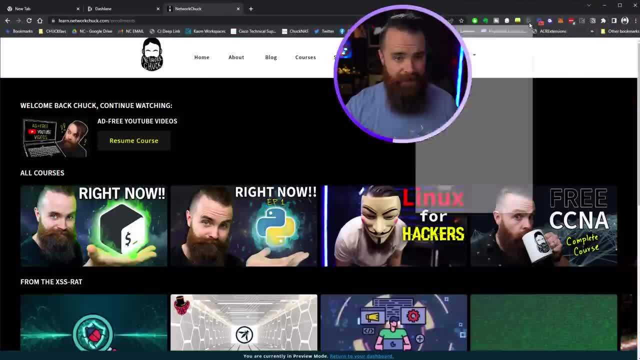 change your dang password. And then, right here is my favorite feature of Dashlane: It's got two factor built right into it. So to log into network, Chuck Academy, I've got my security code right here. Oh, don't copy that, Now it's going to change. 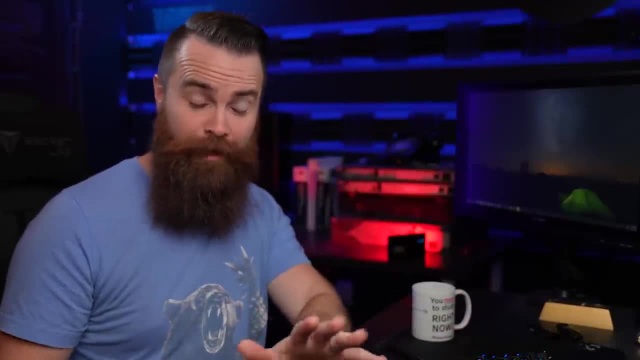 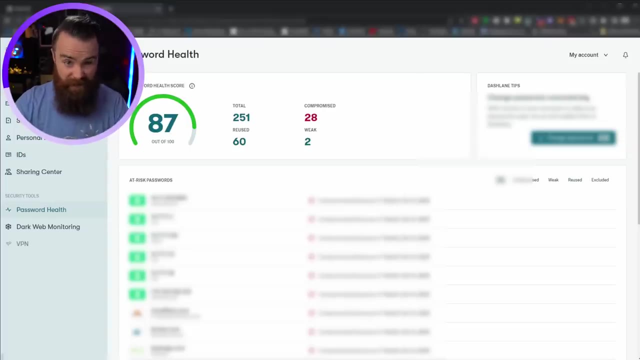 So I pretty much use Dashlane for everything, including my business. I force all of my employees to use Dashlane because they're crazy and they still write their passwords down on post-it notes, Come on. So if you have a business, use Dashlane. they've got a great admin section. 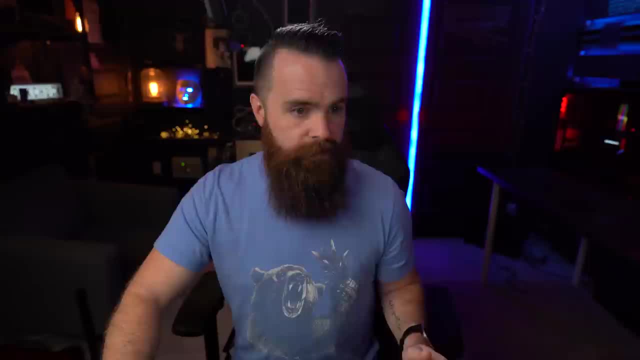 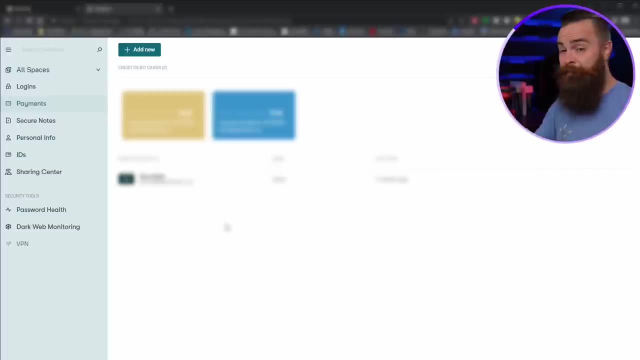 It's a little admin console where you can manage all your passwords for your employees. Got to keep them suckers in line, And it's not just passwords. You can put secure notes, You can put your payments in here. I use this all the time. It makes paying for things so much easier. 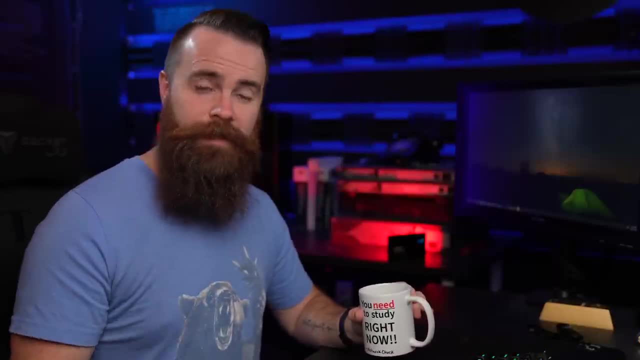 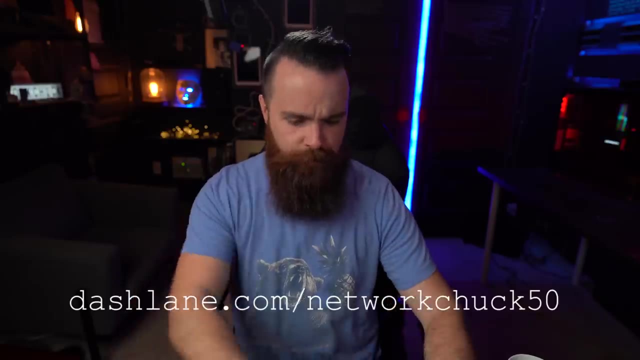 So don't let someone else's bad database put you at risk. get yourself the password manager. I recommend Dashlane. go out to Dashlanecom, forward slash network Chuck 50. And you do get a discount. Let me double check what that is. I forgot. Oh sweet, You get 50% off. 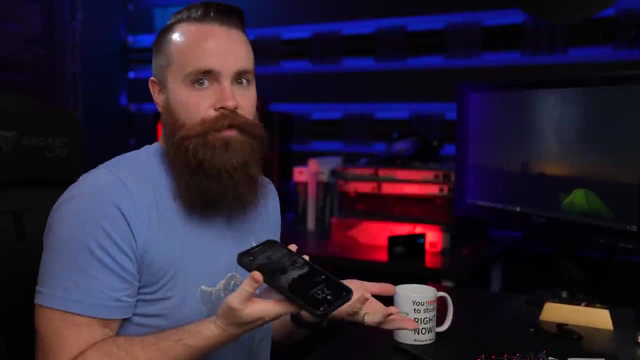 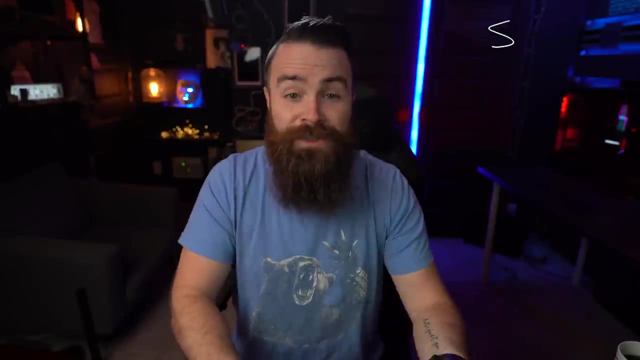 So use that code. You can use it on pretty much Any device you have, which I do on every device. Thank you to Dashlane for sponsoring this video. Now let's get back to SQL. Here we go. So SQL or SQL. 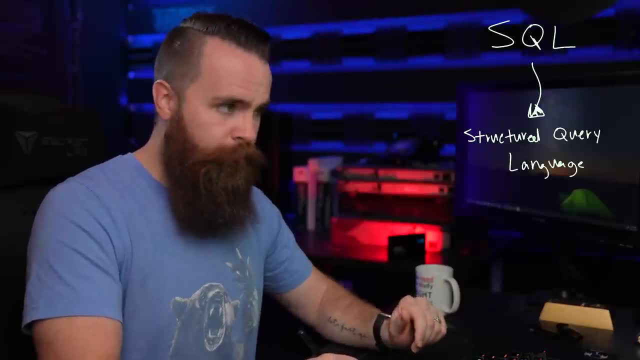 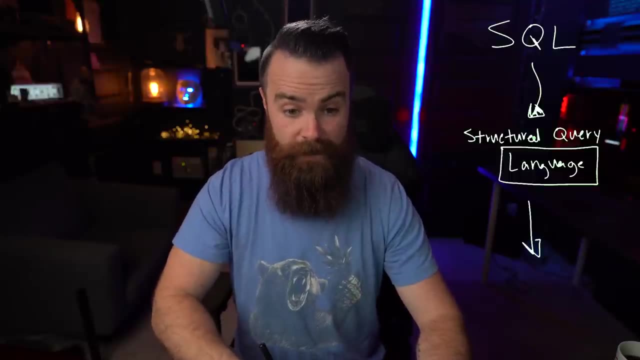 it stands for structured query language, focused on that term language, because it is kind of like a programming language similar to Python, except the primary use of SQL is to talk to databases. I told you it's their love language. They love it. That's my database, by the way. 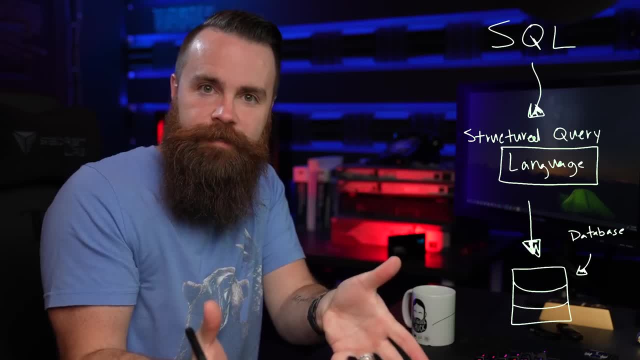 I'm going to label it using this query language. We'll talk to our database. We'll create things. We'll read things. We'll update things. We'll create things. We'll read things. We'll update things. We'll delete things. Crud- You've heard of crud, right? Well, you just did. 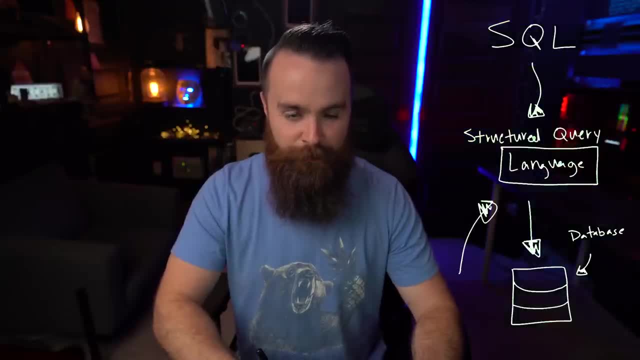 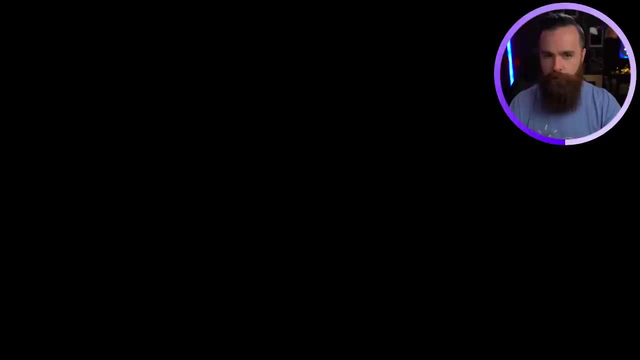 So here we go. We are going to learn some SQL here in a bit, but first let's talk about what's a database. I joked earlier how it's just one big giant Excel spreadsheet. That's kind of true. You've probably seen an Excel spreadsheet before, right. 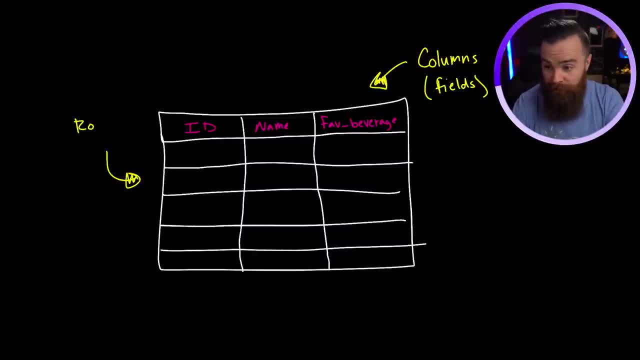 It has columns or fields, It has rows, or we might call those records, and these rows or records contain our data. And while Excel might work for Karen the accountant keeping track of your budget, you bought 45 raspberry pies for bigger sets. 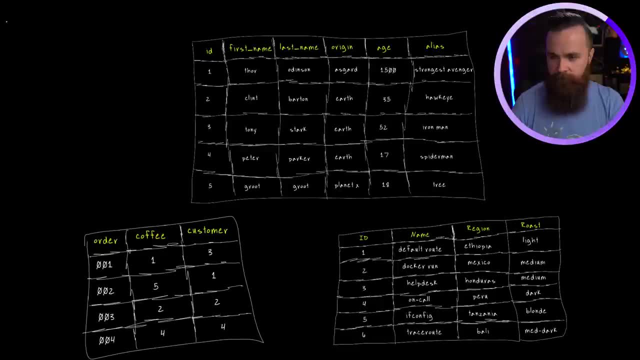 Of data, like websites might have companies, even network Chuck coffee. They won't store these in Excel. They'll store them inside a database which will function very similarly to an Excel spreadsheet, Cause we're still working with this- which we'll call a table. 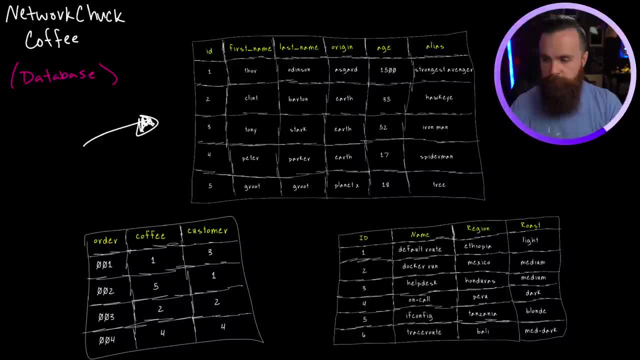 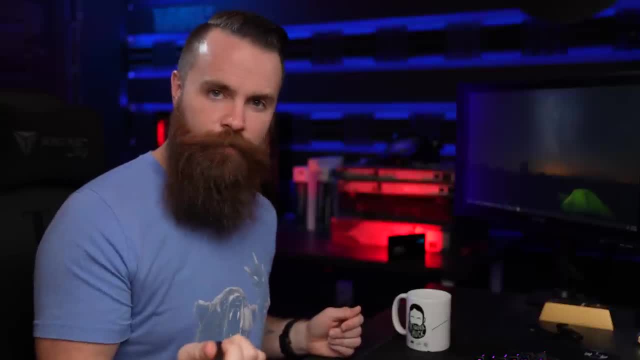 but we might need more than one and we might need a lot more data. So in my network Chuck coffee database I might have three Excel spreadsheets or three tables, one for all my customers. which did you know that Marvel characters love my coffee? Thor can't get enough of. 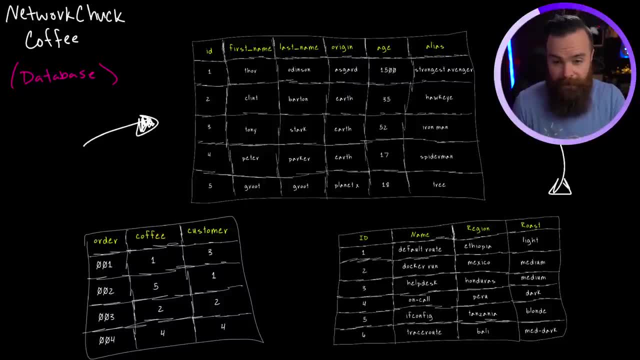 the help desk. He loves it. And then I'll have a table of all the coffees I offer And then, of course, an order table tracking all the orders that are placed. And this is a very, very small, abbreviated example of all the data, my network, 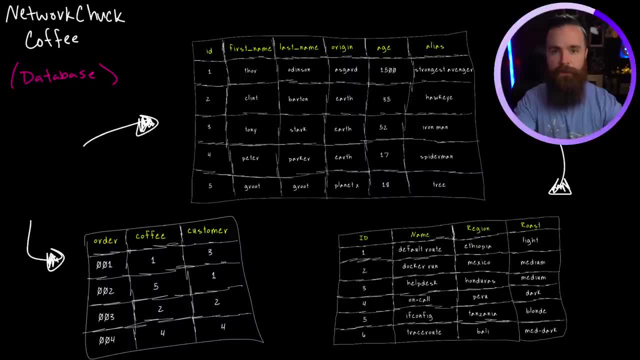 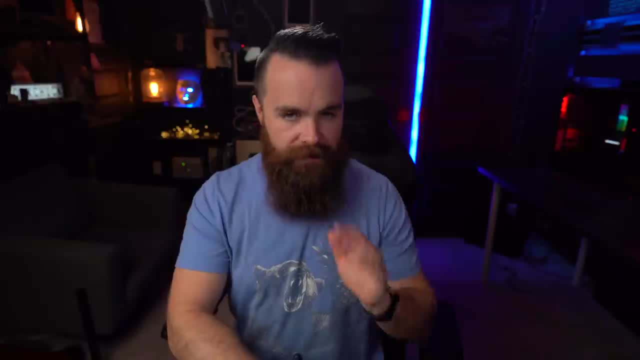 Chuck coffee database might have, which it does have. So the takeaway here is that databases are used to store large amounts of data, data that Karen and her spreadsheet in Excel couldn't even dream about. Now, these databases, they need a manager. 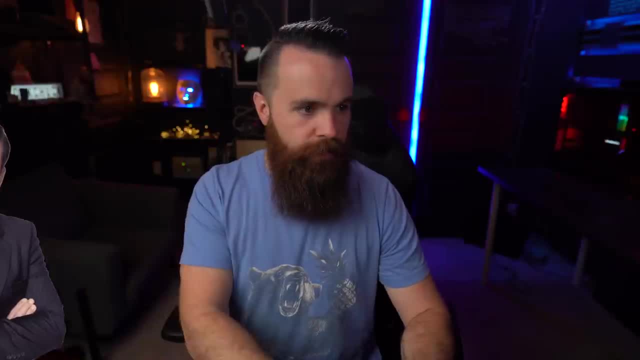 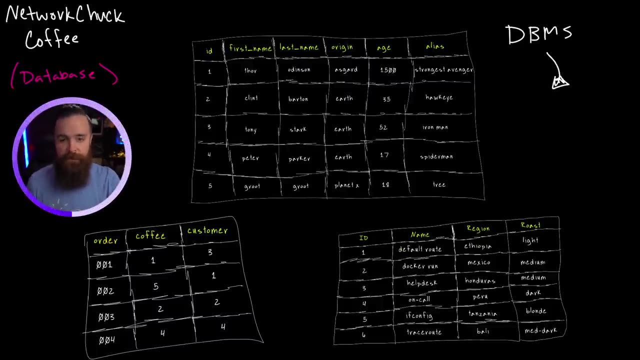 They need someone to control them, to get them in line, Cause they can act pretty crazy if they don't have someone watching them. That's why we have DBMS, a David Bumble management system. No, I'm just kidding, I've been picking on him a lot in this video. Love you, David. DBMS stands for database. 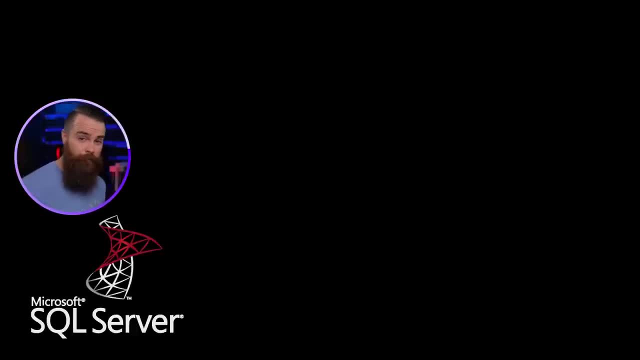 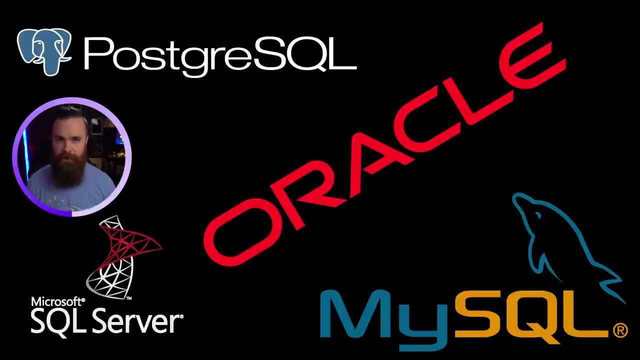 management system, And actually you've probably heard of a few of them: Microsoft SQL server, my SQL or, I'm sorry, my SQL, get post gray SQL. Am I saying that right? I don't know. Oracle, There's a lot out there. 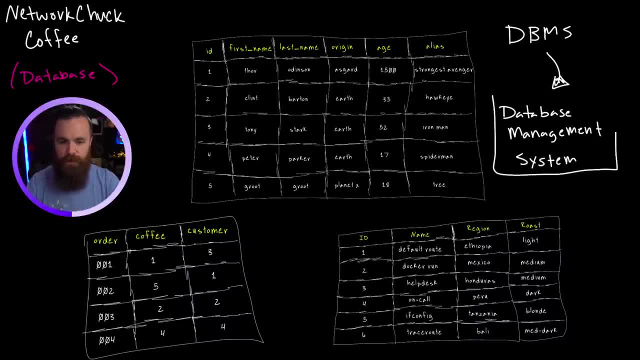 but just know that whatever DBMS you choose, whether it be my SQL, SQL Oracle, whatever their job is to manage your databases, They will have different ways they do that, but they're all going to use SQL, the structured query, the- I can't even say it- structured query language. There we go. 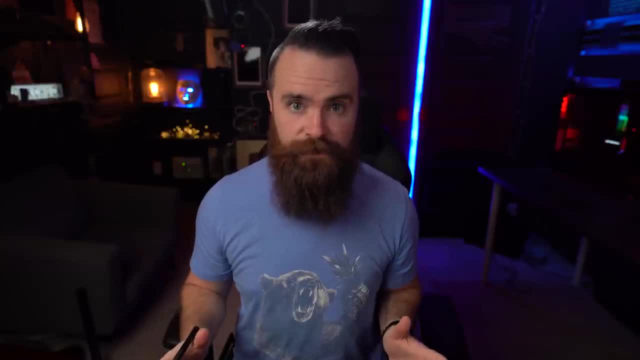 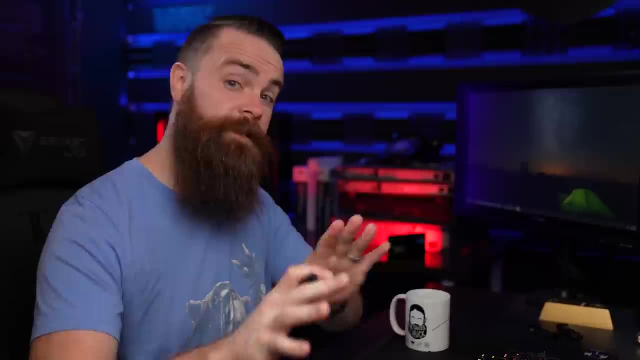 10 times, 10 times fast on that one. This is actually a standard that's been ratified by the ISO, ISO. So if you learn SQL, you can pretty much approach most databases with relative ease. Now there are some nuances, some differences, going from like Microsoft SQL to my SQL. 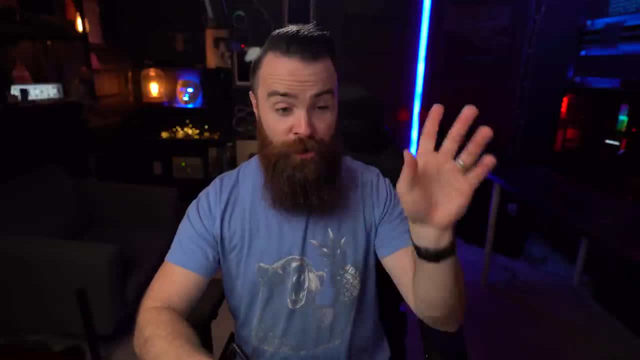 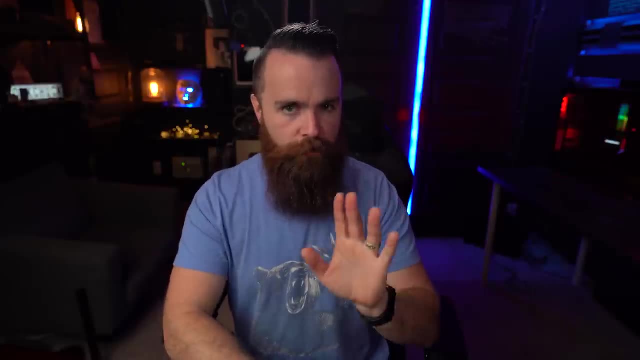 but it's nothing you can't Google as long as you understand the concepts. Now, just so you know, we're going to create these three databases ourselves. We're going to install one and actually make it happen with my SQL, But before we do that, there are two database types. You have to know about this. 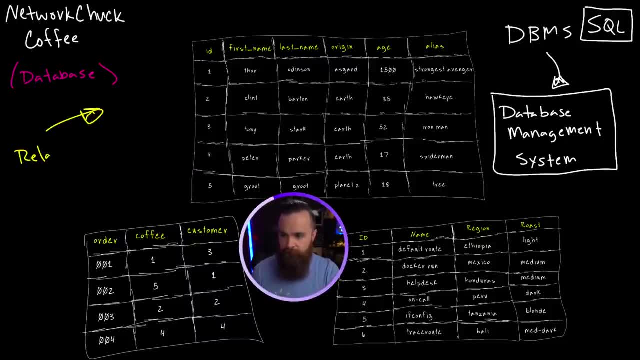 When we're talking about here. this is a relational database. You might see it abbreviated as RDBMS, and they by far are the most popular. It's what I drew out here And what makes it relational is these tables here kind of like they're related. 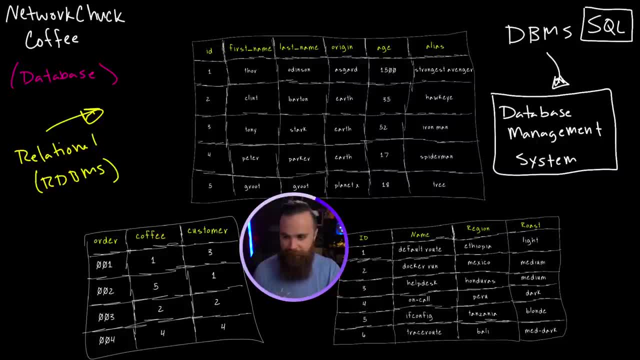 They're cousins or brothers, I don't know. They're in the family. And what I mean is like when in this table, here on my orders table, it says for order zero zero one, the coffee was one. And you're like what is? 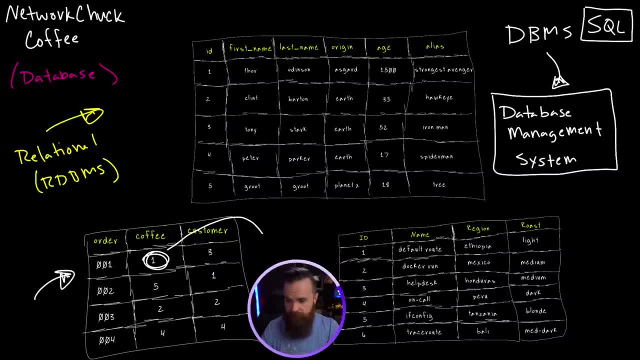 what does that mean? Well, it's actually tying back to the coffee database. And then when it says customer is three, you probably guessed it's looking back at the customer database saying, Hey, Tony Stark ordered the default route. He loves that stuff. Now again. 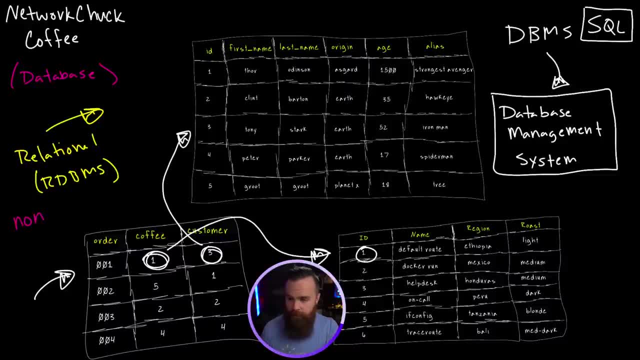 we're gonna zero in on the relational database, but the other type you wanna know about is the non-relational. This one doesn't have any family or any friends. He's very sad. We're not gonna cover what it is here, but one type or one DBMS you might hear about is no SQL. 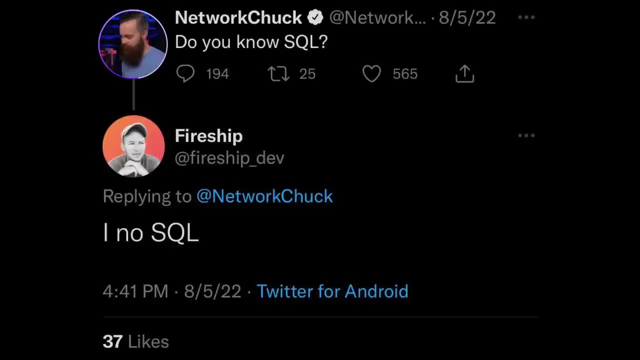 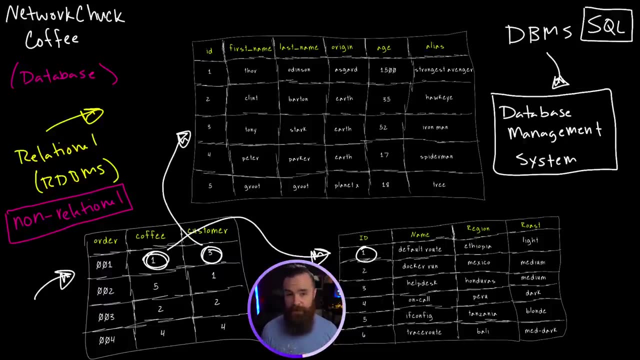 which Fireship did a great joke on Twitter When I asked you guys if you know SQL, well played, sir. but a non-relational it's not like this. It's not related, It's kind of unstructured data and it definitely has its use. 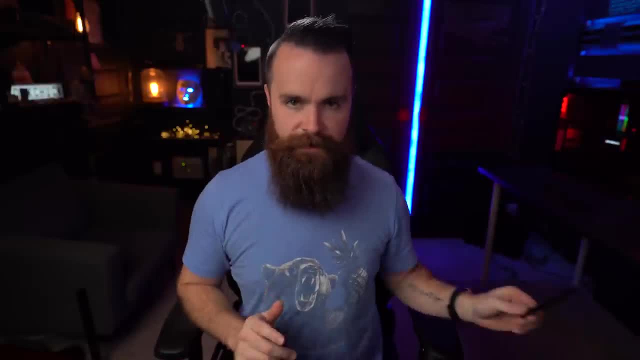 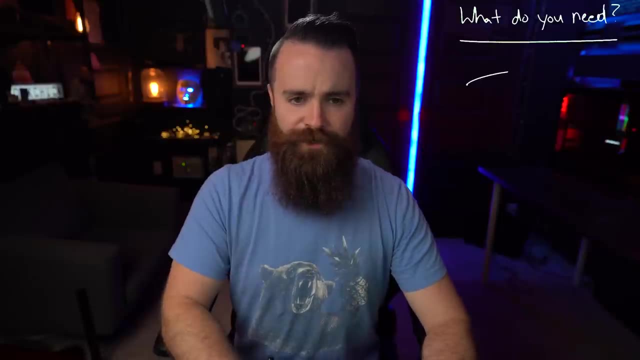 case and purpose, but we're not gonna cover that right here. Okay, Enough about databases, Let's actually make one right now. It's completely free and completely fun. Now, here's what you need. You won't need much, pretty much any computer, That's it. 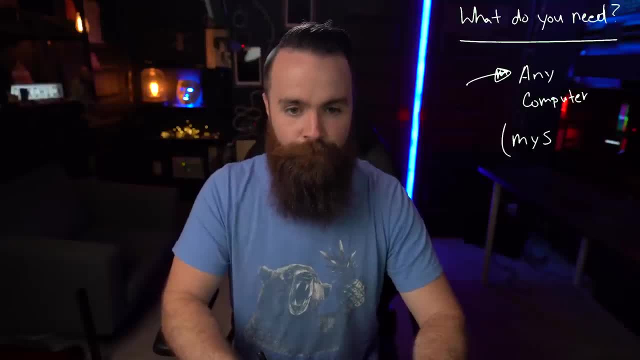 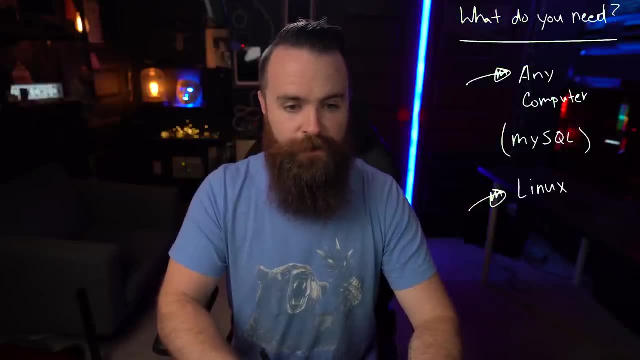 We're gonna be playing with my SQL or my SQL, and you can pretty much install that anywhere for free, including windows. Now I will be walking you through Linux, because I love Linux and it's so easy. So if you wanna follow along with me exactly from the beginning, 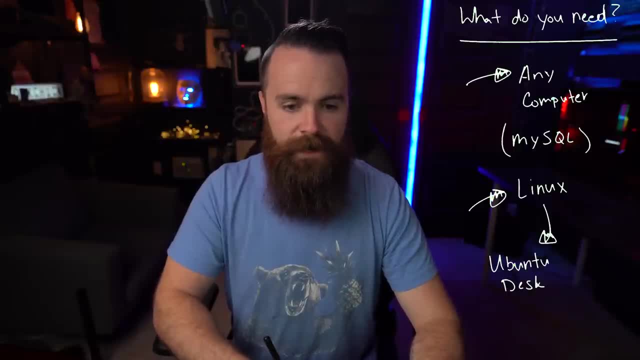 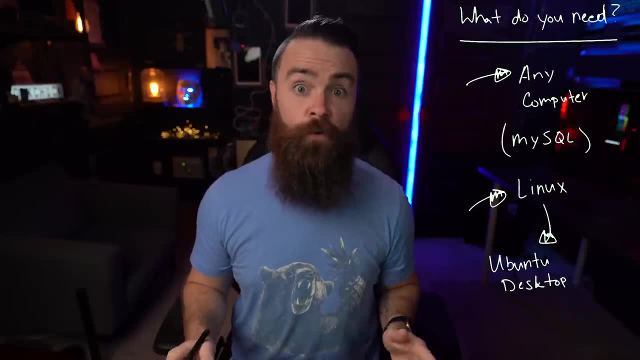 from the start. I'm gonna be running the latest version of Ubuntu desktop inside a virtual box VM. If you're like wait, what, what, what's he doing? I've got a video right here on how to set up virtual machines and what they are. 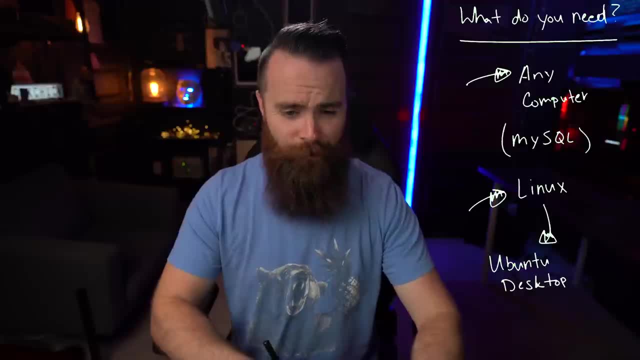 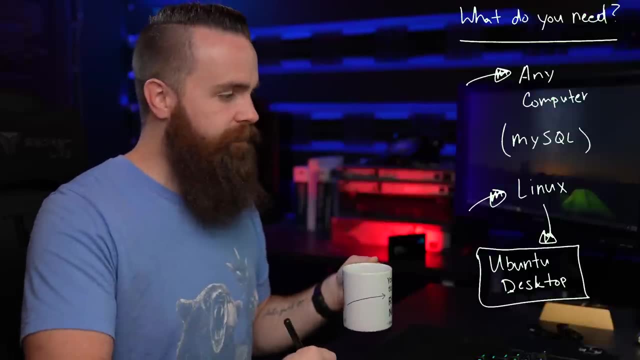 and why they're incredible. You should go watch that if you haven't already. And it's completely free to run this. And yeah, that's it. Oh, I forgot, You need coffee, because everything in it it requires coffee network. 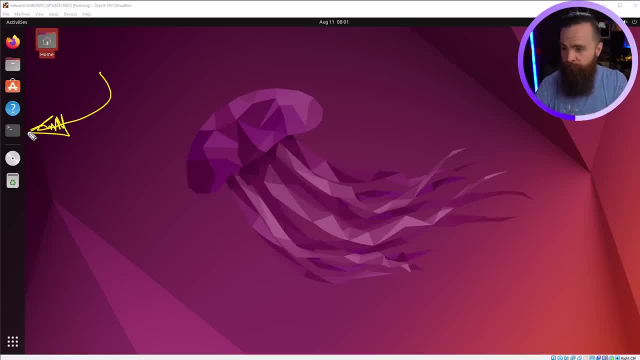 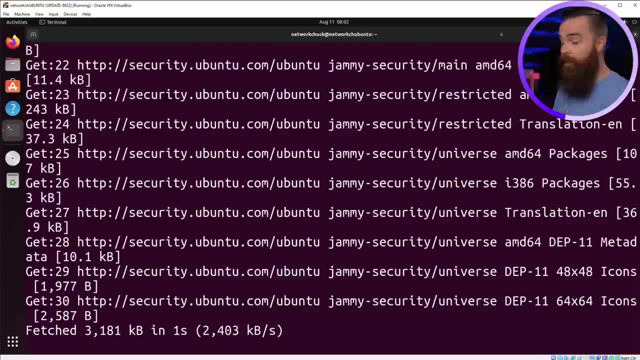 chuckcoffee. So here in Ubuntu, we're going to launch our terminal first. Like always, we'll get our repositories updated- pseudo APT update and quick Step A Coffee while it does its thing. Next, we'll install SQL server with one command: pseudo APT. 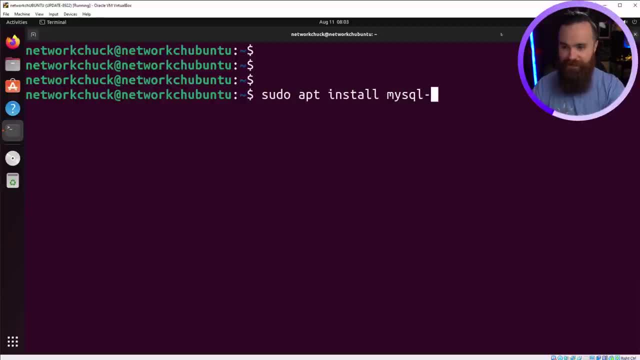 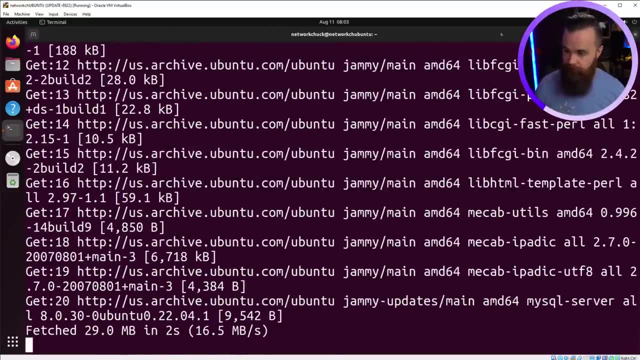 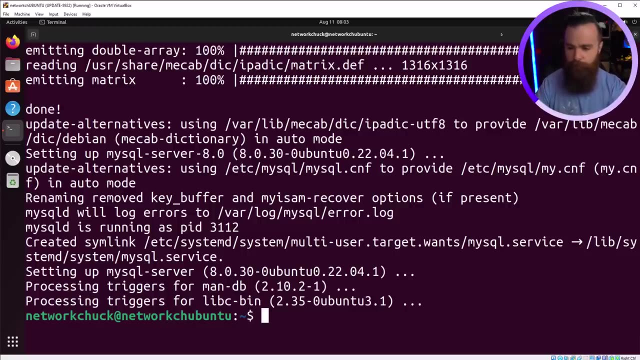 install my SQL dash server. We'll do a tick Y at the end And that's it. It'll take just a few moments, and perfect time for a coffee break- We can never have too much. Now, at this point you're pretty much running my SQL. Let's verify it real quick though. 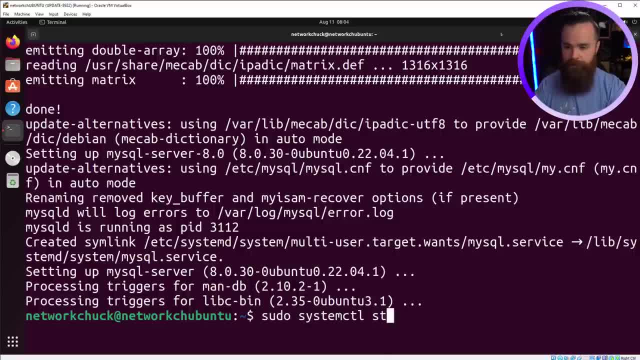 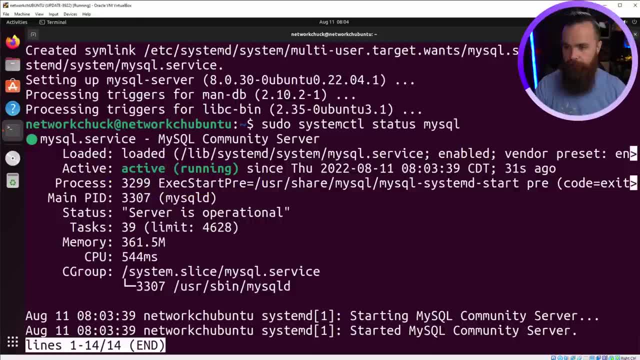 Let's make sure the service is up and running. We'll do a pseudo system, CTL status, my SQL And fingers crossed. You should see active and running. That means it's healthy. Good to go And just hit Q to get out of there. 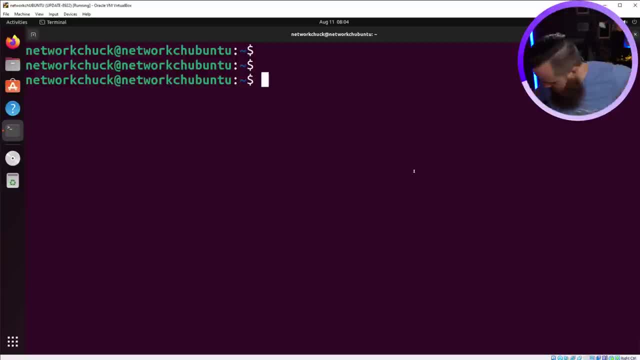 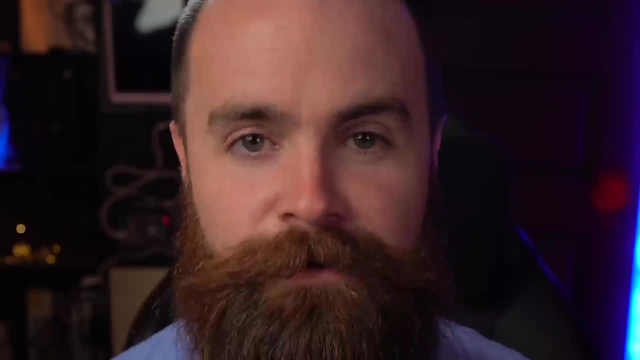 Now go ahead and play with your database. Just go crazy. You're like: wait, where is it? to access it, All you have to do is type in my SQL. That's it. Well, not it. You're going to have to do pseudo my SQL. 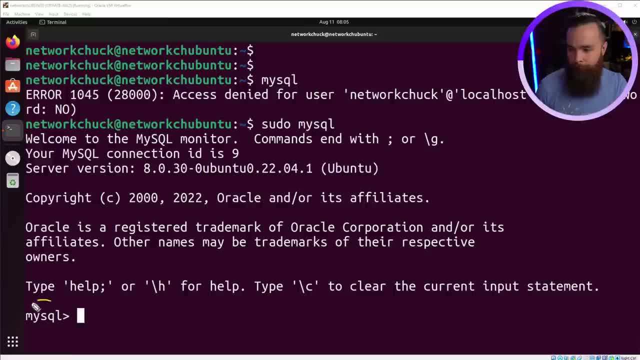 Let's try it now. Yeah, we're there. Look look at that. We got a nice little my SQL command prompt down here Just waiting for us. The cursor's blinking, ready to go Now, just so you know, the command my SQL, without any parameters at all, worked. 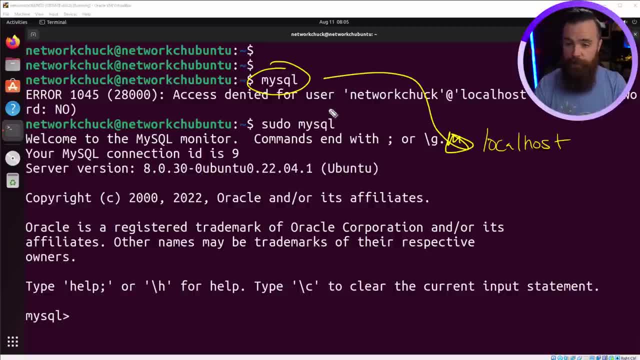 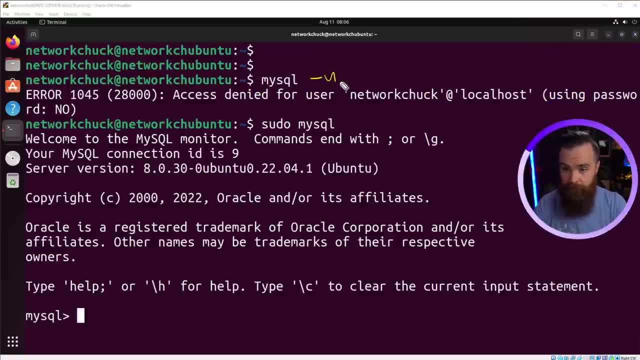 for us because we're connecting to our local host. It also worked because we don't have a password set, which is fine for us as we're just playing around. But often you might see something like this: specifying a username, a remote server you want to connect to the port and then saying dash P for. 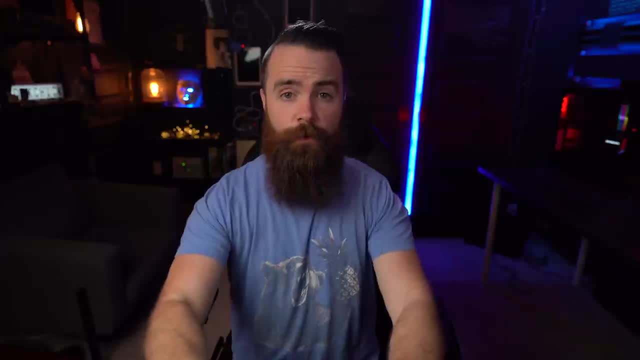 password. But we don't have to do that here, So we're not gonna worry about it. So here in SQL let's get the lay of the land first. What's happening right now? We'll first do a show. databases command Now, just know. 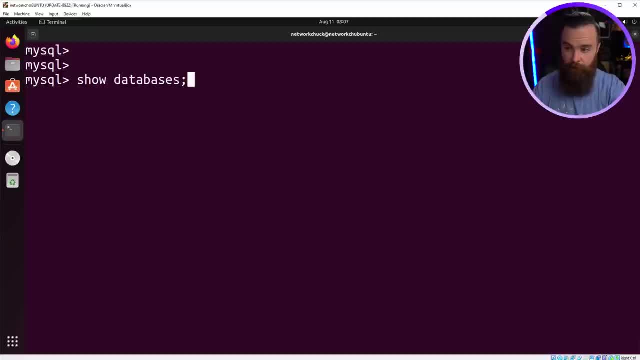 every time you type a command in my SQL, you have to end it with a semi-colon, Otherwise it's like what you're not done yet. Come on So do that And boom, some good old default databases. What do you say? We create our own. 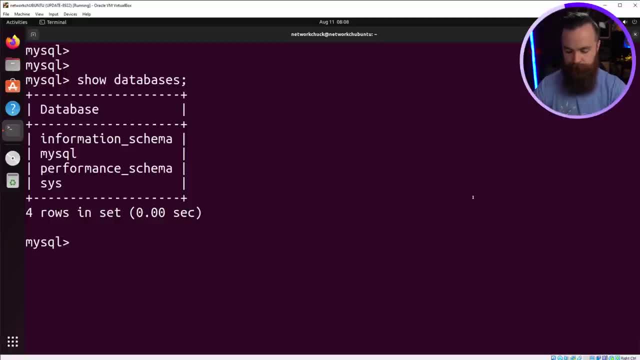 Let's do that right now. We'll create the database for network Chuck coffee. This one's very hard, I'm just kidding, It's gonna be so easy. Simply type in create database, the name of your database, which we'll name, and see underscore copy, and then 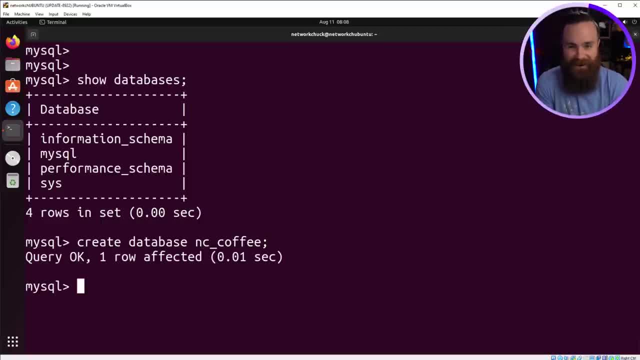 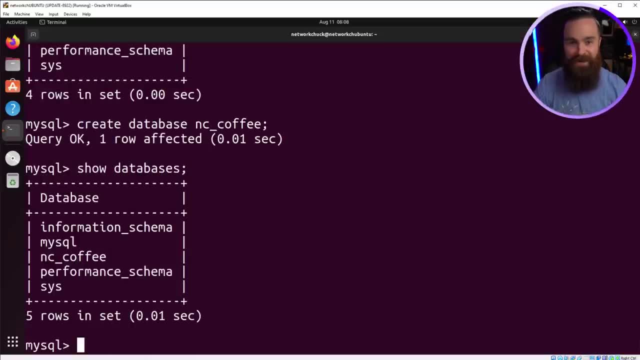 semi-colon Done. How hard was that Right? You just created a database. That's awesome If we do show databases once more there. it is our very own database. but he's just sitting there doing nothing. He's got nothing going on. Let's change that now to play with our database. 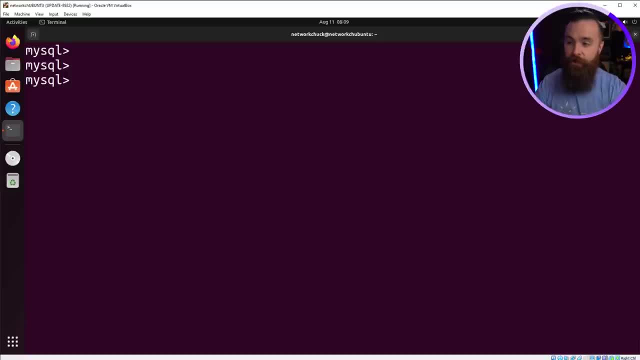 to do things with it, to use it. We're gonna type in the command use and then the name of our database and see underscore copy semi-colon. And that's it: Database change. Now we're interacting with that guy right now. Now, remember a database. 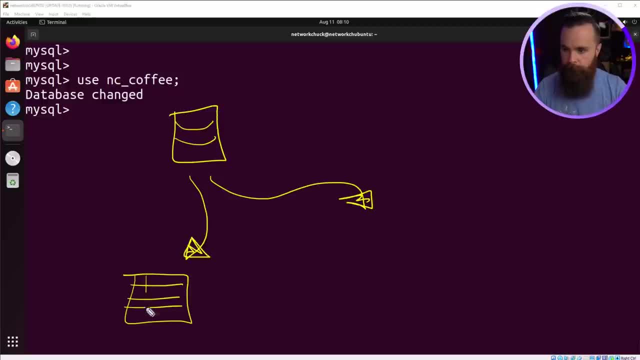 we'll have a bunch of tables, assuming you created them, but right now ours won't have any, and I can prove it to you. Let's type in the command show tables. the semi-colon empty set nothing there. So let's change that. Let's create our first table. 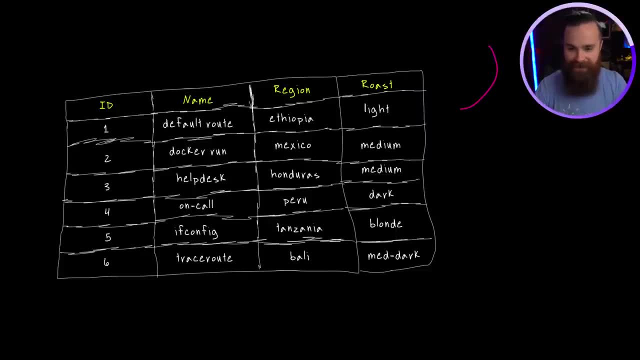 And this is so cool. This is gonna be fun. The first table we'll create is our coffee table. but um, and right now, I want you to just ignore the rows. Don't worry about the rows, the, the data, all right here. All I want you to focus on are the columns ID. 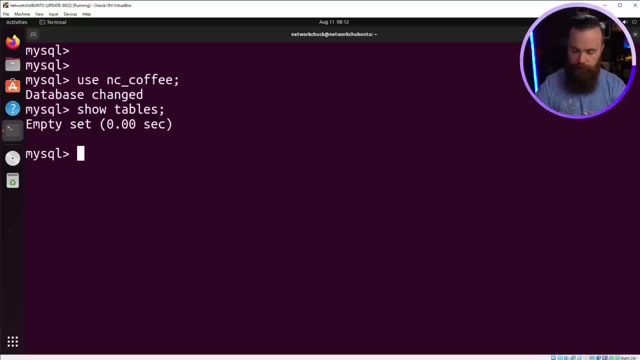 name region and roast. We're gonna deal with that right now. So to create a table, we're gonna type in create table, crazy, right. And then right after that we'll name our table. Of course we gotta name it coffee table. Don't wanna miss that opportunity. 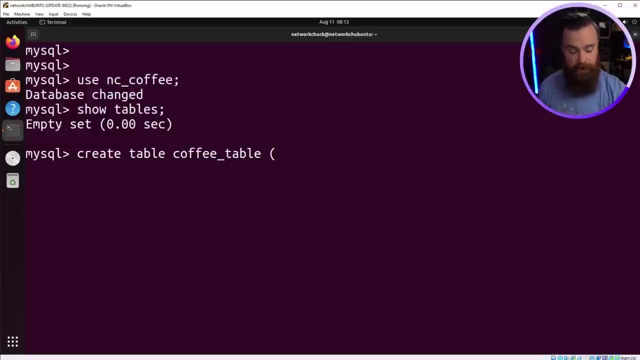 And then right after that, we'll do an open parenthesis and go ahead and hit enter. It'll be fine, because we didn't put a semi-colon. semi-colon means you're done. doing anything else means like I'm not done yet. That's, that's what it means. 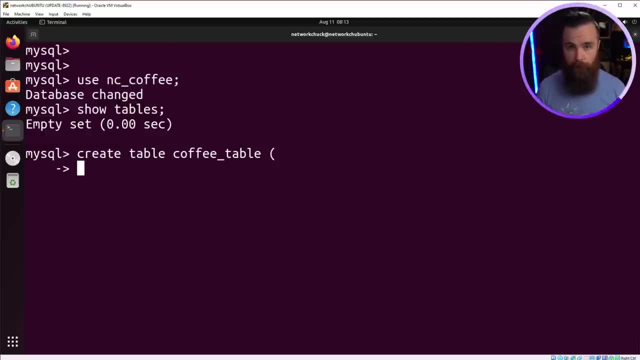 Now here, inside these parentheses, we'll be defining our columns. What we saw before: ID name, blah, blah, you know you got it. So our first column we'll simply call ID And then, right after that, I'm gonna type in: I N T. 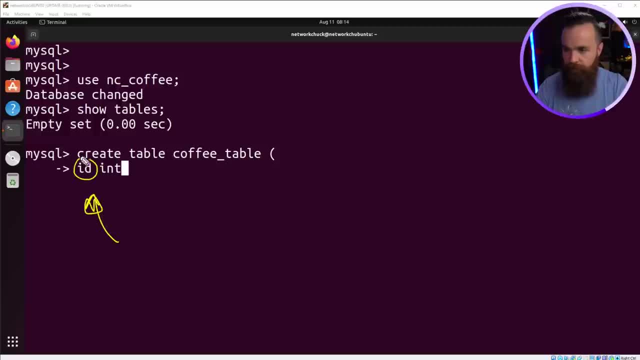 Now what is that? So here's our column. We're defining the name of our column- that guy right there- But then we also have to define what type of data is gonna be in that column or in the rows that we're gonna have underneath it here. 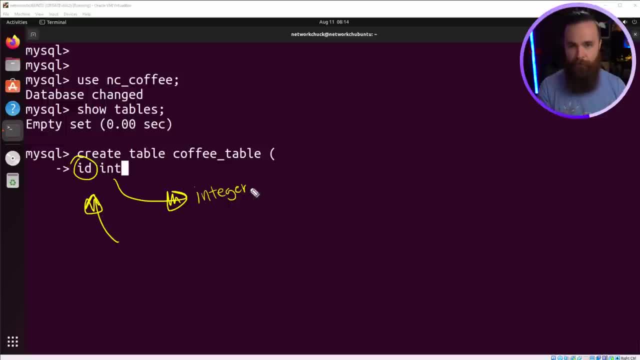 We're saying we want it to be an integer or a number. That's the type of data that will live in that column And that's pretty much all there is to it. We'll type in a comma to tell them that Hey. 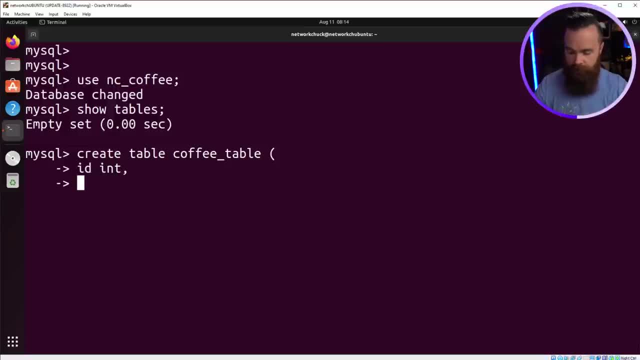 we're not done with our columns just yet. Hit enter Our next column. We'll be named and then we'll define what type of data we want inside that column. here I'm gonna type in V A, R, C, H, A, R or variable character. 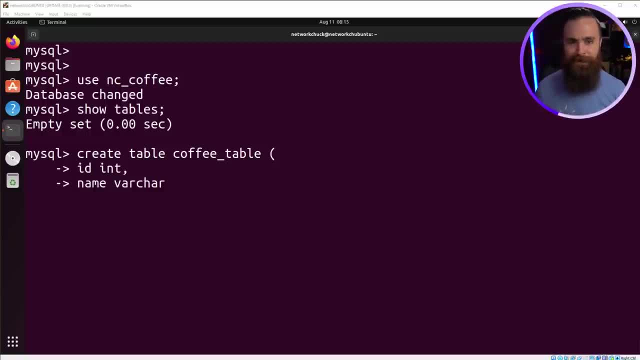 which is an indeterminate length string data type. Basically it's just letters and stuff. It's a string. I can also define how long I want that to be, how many characters are allowed. So I'll just say 255 in parentheses, just like that. 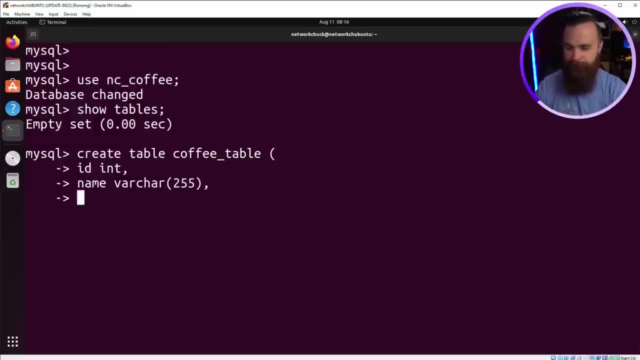 And let's keep going. comma next thing, Or column, It was region. This will also be a string or variable character, and we'll keep going until we're done. Oh, we only have one more roast. Now my last column. here I'm not going to add a comma. 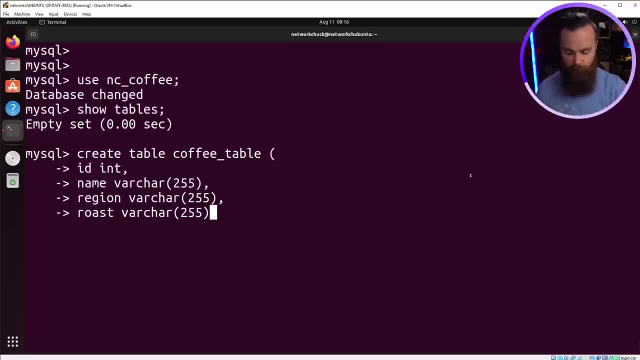 You only add a comma when you're saying, Hey, I have more to say, We don't have more to say, we're done. I'll hit enter, I'll do a closing parentheses And then to end our command, like we do in all my SQL stuff, we're gonna type in a semi colon. That's it. 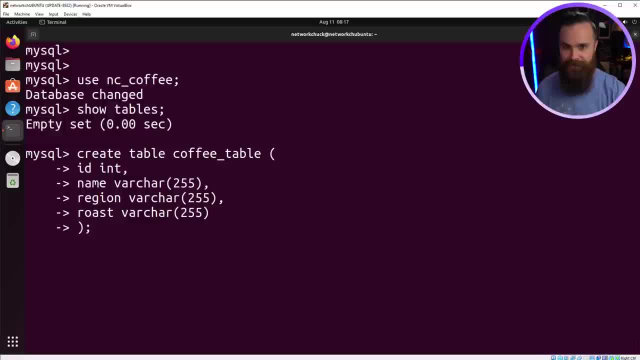 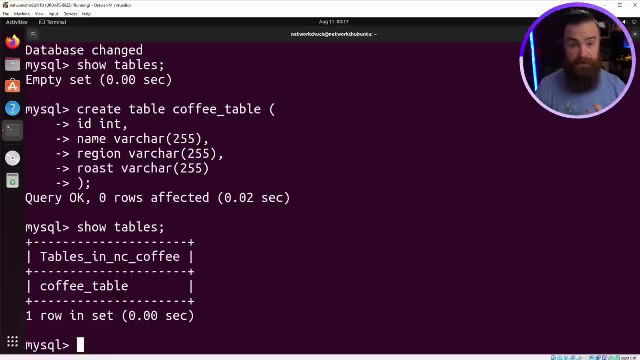 We're about to create our first table inside our database, Ready set, enter, go. Let's take a look at it. Show tables. There it is. There's our coffee table. Now, that's just the name of it. What do you say? We look inside and see the actual columns we made. 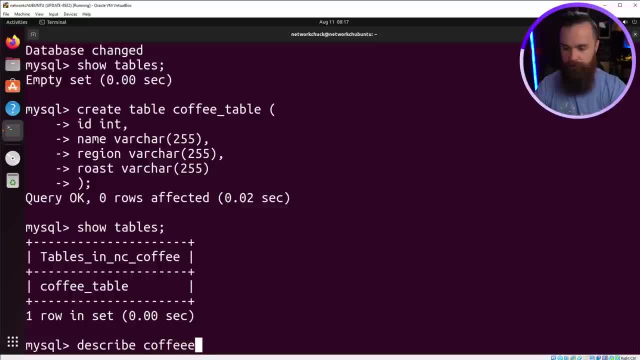 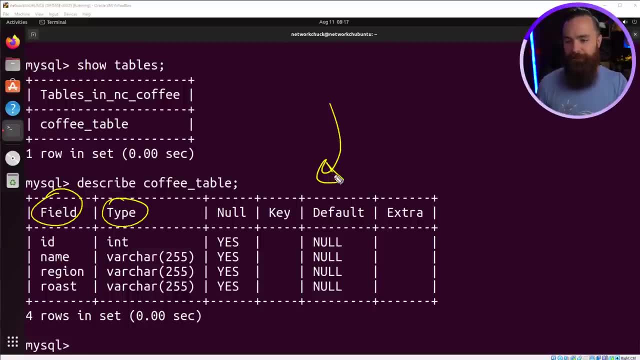 We can type in describe coffee table and that'll give us some more info. We got our field and our type and we'll cover more on this stuff here in a minute. Oh and, by the way, when we're defining our table and defining that columns and everything. 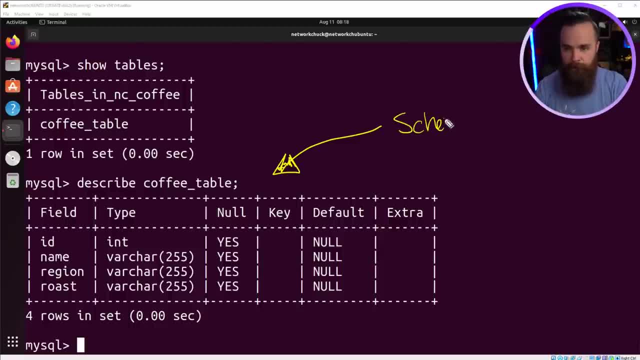 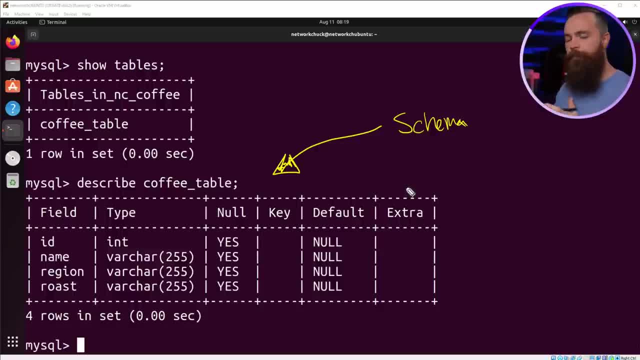 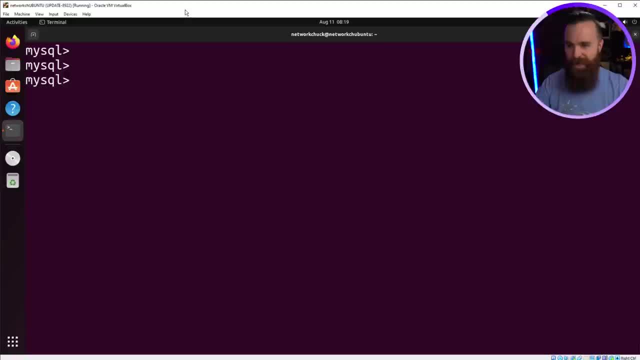 Looking at our database, let's add the default route. Let's insert a row into our table and my SQL. we'll type in insert and two and then we'll specify our table, which was coffee table. Then we'll say: here are the values. 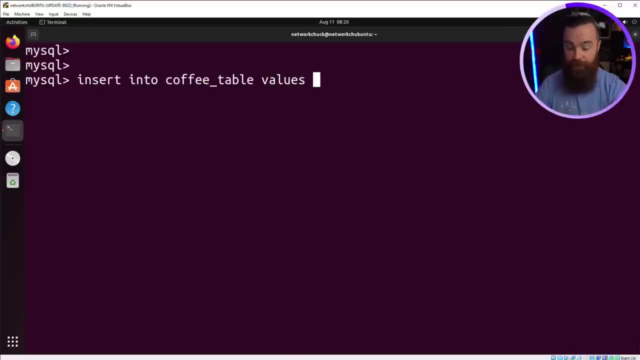 We'll actually use the word the command values, and we'll define our values inside parentheses. The first one's an integer and I'm just gonna put it in as one. that's the first ID. Second one was name, which will be a string, default route. 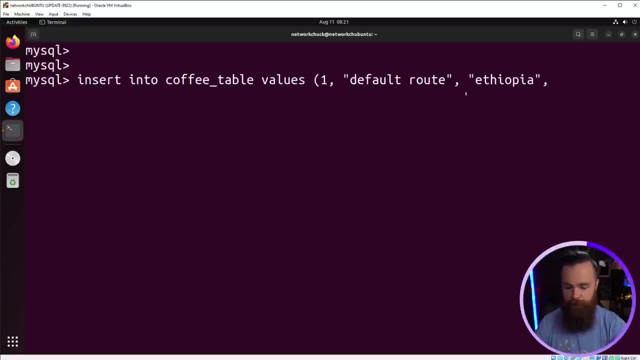 Then origin Ethiopia, also a string And finally roast, which was light. So what's happening here? We have the insert into command, So we're telling MySQL, we're inserting into the coffee table table And it's like: what are you inserting? 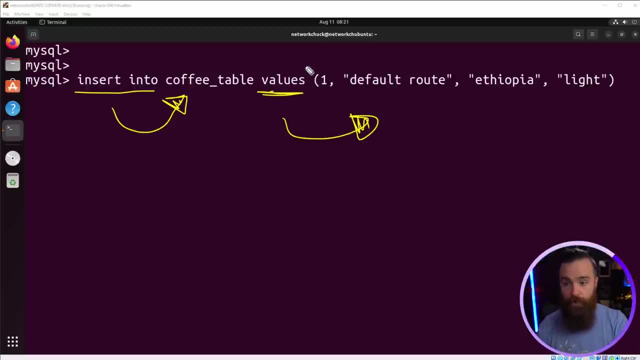 Well, here are our values. bam And notice we're going in order of our columns And we have to do that. Got the ID, the name, the region and the roast. Then, once we're done, what do we do? 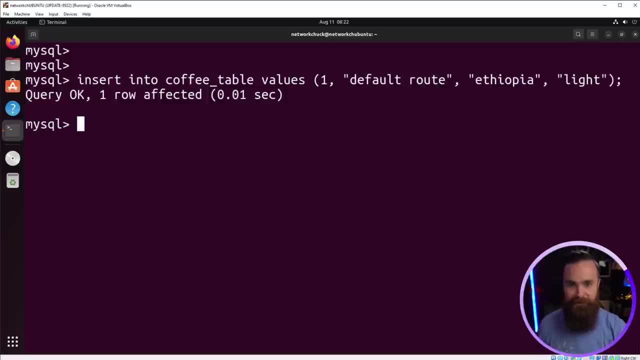 We type in semicolon to say we are done and awesome. Now what I love about MySQL and most SQL things is it'll tell us, hey, the query it's okay, We got this, it's good. And it tells us there was one row affected. 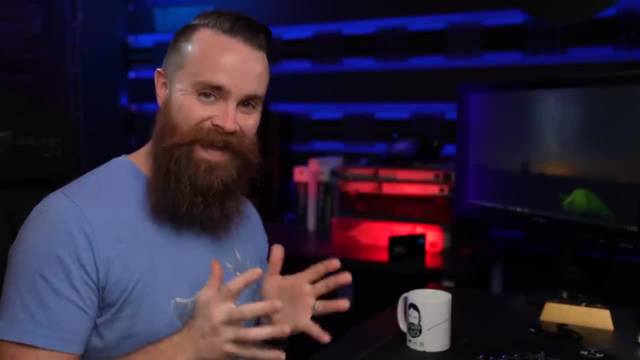 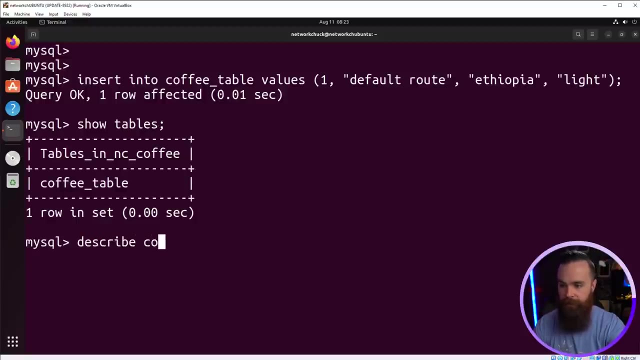 Which row? Well, the one we just added. Now, I know you wanna see that data inside your database, but so far I haven't shown you how to do that, Cause if we do show tables or describe coffee table, it doesn't show us the data inside yet. 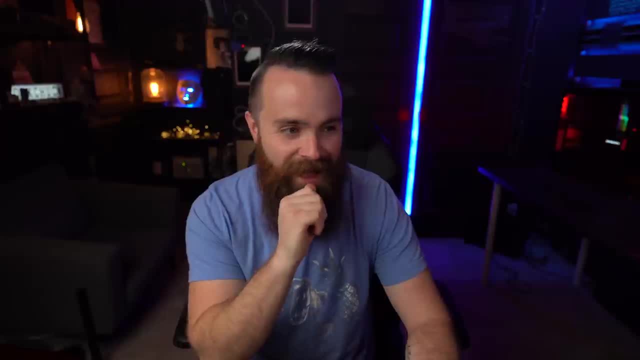 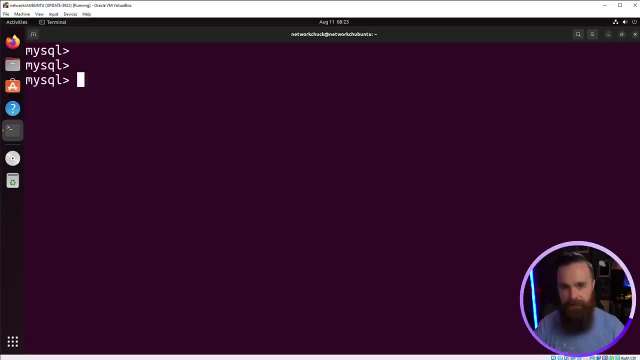 So I guess I can go ahead and show you your first select statement. Ah, should I wait? Yeah, no, let's do it right now. I know you can't wait. So here's how we look inside of our table. Let's pull some data out of there. 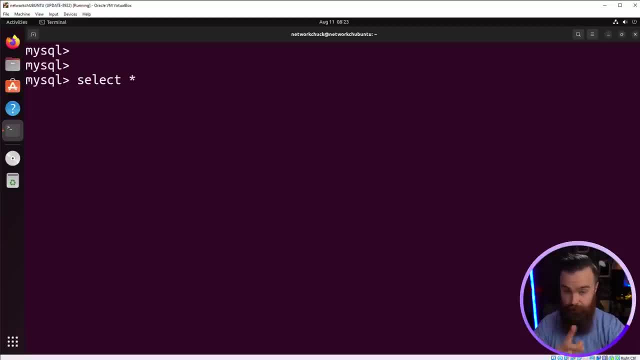 We'll type in select, we'll do an asterisk and I'll explain this here in a second And we'll say from our table: coffee table, semicolon. Now what's happening here? Well, I wanna select some data. 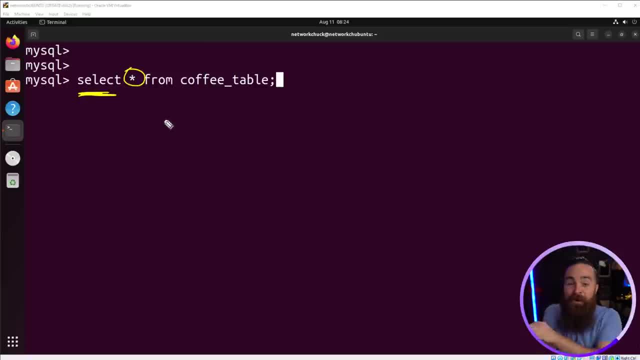 And it's like: well, what data From what column? And we're saying all of it. I want everything. That's what the asterisk means. And then it's like, okay, fine, From what table? Where are you getting this from? 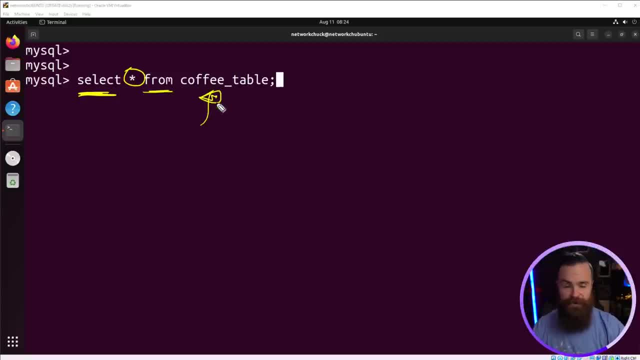 Well, we're getting it from our coffee table. I wanna see my coffee stuff And that's what we're doing here. It's a very basic select statement. You'll see this one all the time, But if you just wanna pull all the info from a table, 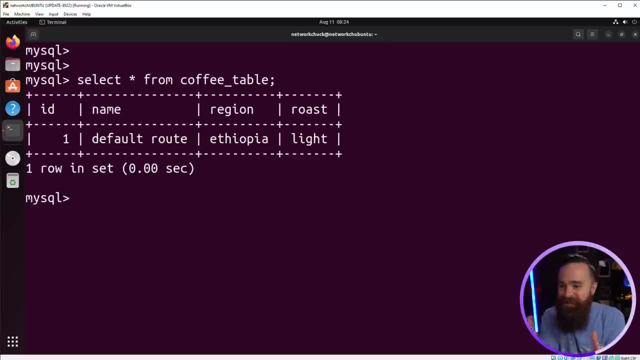 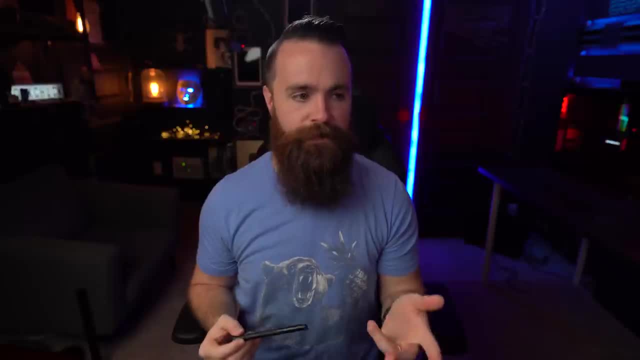 that's how you do it. Let's take a look There it is. How cool is that? So if you just did this, clap, pat yourself on the back, That's a big deal. You created a database. you created a table inside that database. 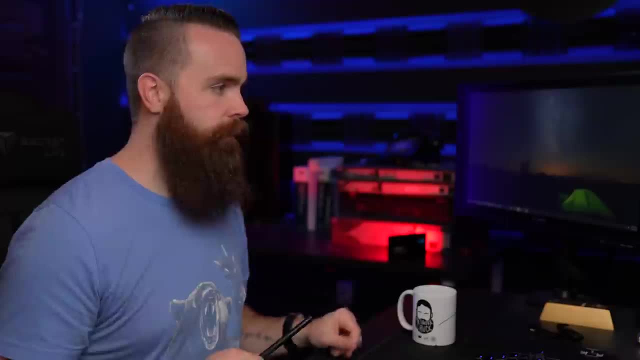 and you added some data to it. Simple, but killer. Now here's a challenge for you. What I want you to do is fill out the rest of this database, All the rest of our coffees. Go ahead and pause the video. 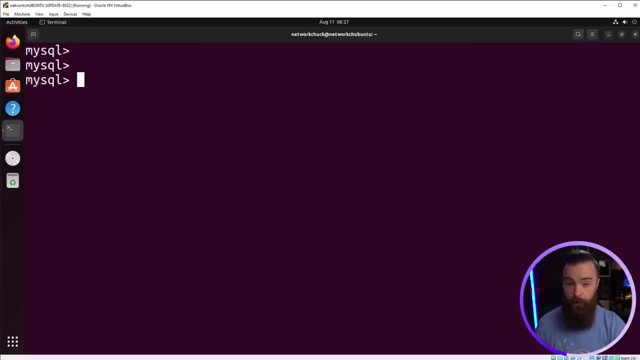 Pause, Unpause. Let's see how you did. Let's do our select statement once more: Select everything from coffee table, And we should see a lot more things. Yes, it's so nice and neat. I love it. If yours looks like this, congrats. 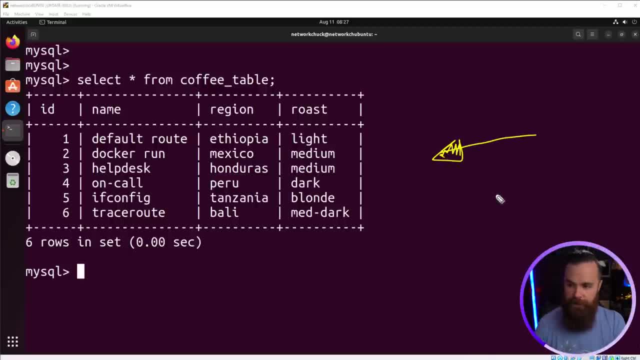 That's awesome. Now another challenge for you: I want you to select only the names of the coffee from that table. That's all I wanna see. Can you do that? Let's try it out. Select Instead of saying everything. 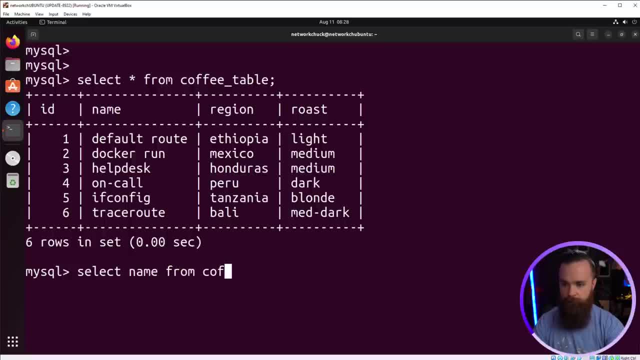 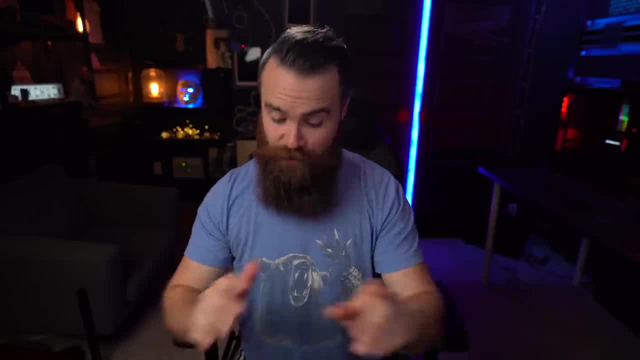 let's just select the name from coffee table. Bam just got the names of our coffee. That's it. Now here's the next challenge for you. I want you to create our next table And do this by yourself. I'm not gonna show you. 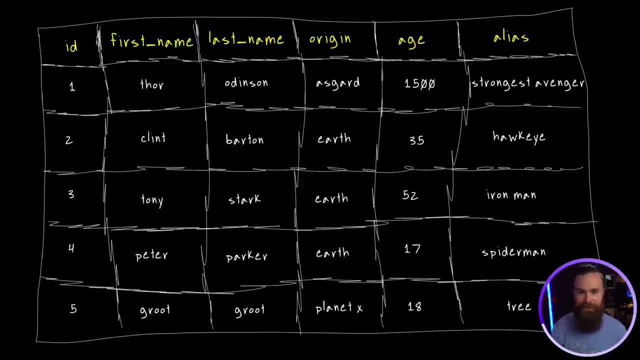 Create our customer table with all of our Marvel customers And also name your table Avengers, Just like this. Okay, pause the video, Go Unpause. Let's see how you did. Now again, I wanted you to create this table. 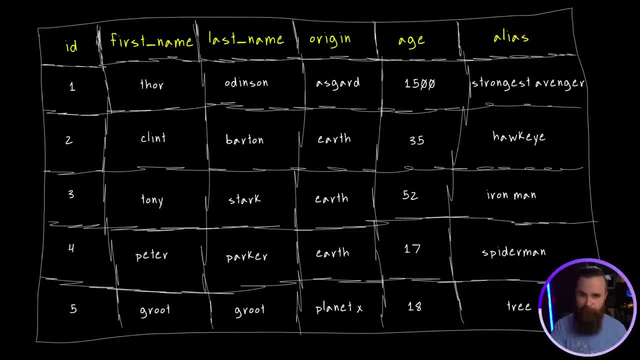 And if you haven't already, go ahead and fill it out with all this information. It'll take about two minutes, but it gives you practice. But if you did it right, it should look like this: Let's go ahead and select everything from that table. 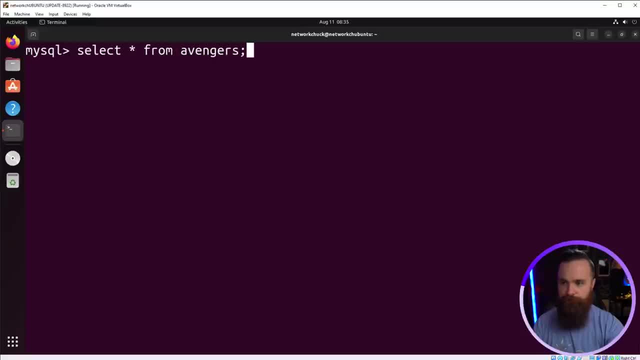 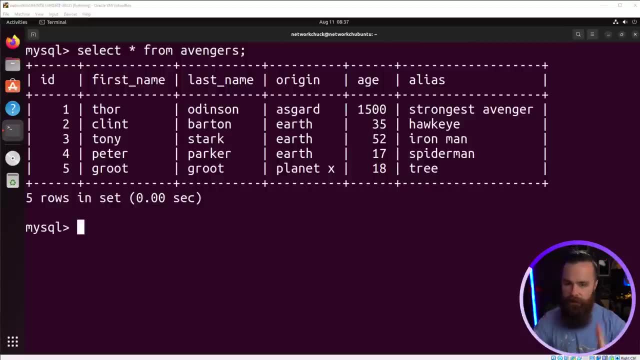 Select all columns from Avengers. Let's see how it looks. Oh nice, clean, tidy data. I love it. Now here with our Marvel characters. let me show you some of the things that you can do Now here with our Marvel characters. let me show you some of the things that you can do. 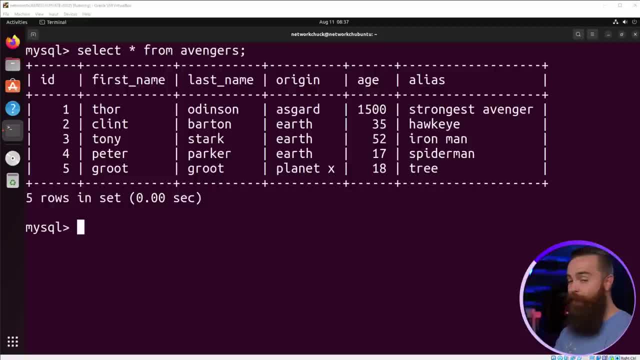 Now here with our Marvel characters, let me show you some of the things that you can do, The power of SQL and how we can find or query our data. So let's try this. Let's do a select statement, just like we did before. 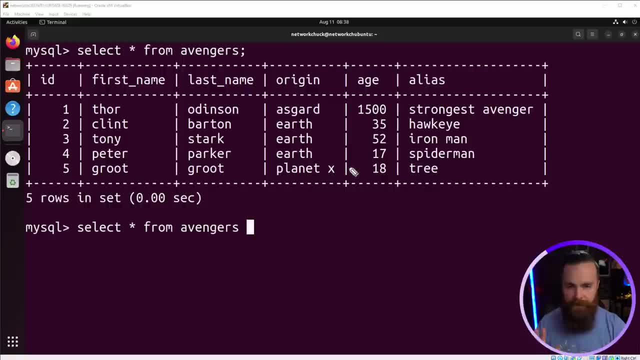 Select everything from Avengers. But let's say we only wanna see the Avengers that are from Earth. That's all we wanna see. How do we do that With where? No, I'm not losing my mind. Watch this. I can add another filter saying where- origin. 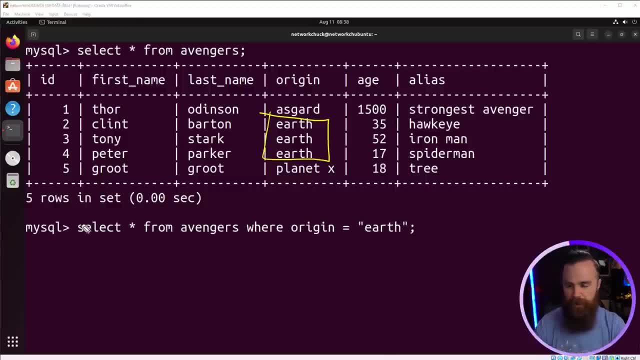 equals the string Earth semicolon. So let's break it down. I'm selecting all columns from the table Avengers, But I only wanna see where the column origin equals Earth. That's it. Let's see what happens. Bam Only got the Earthlings. 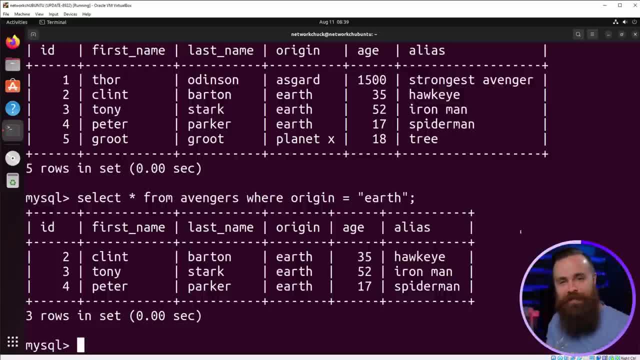 Check it out. Isn't that cool, though, If you had a large amount of data being able to just select, pinpoint the data you want. like that is killer, And that's just a basic SQL statement. Let me show you a few more quick ones. 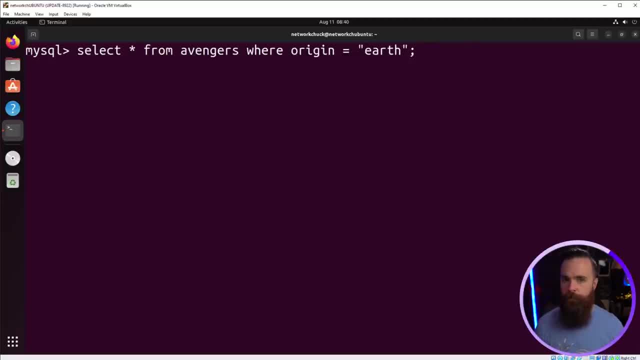 Let's pull up that same statement. Let's say we wanted to see all the Avengers from Earth and Asgard. How would we do that? It's pretty simple actually. All I have to do is add one more filter to it. I'll just say, or. 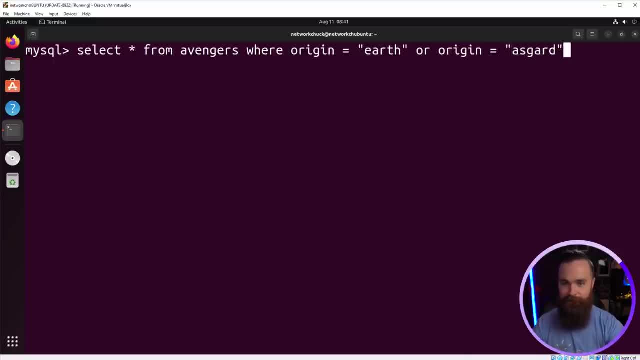 Or origin equals Asgard. So my filter says, hey, origin can be Earth or origin can be Asgard. Let's see what happens. Bam just added Thor, Let's try this one. Maybe I wanna see all the Avengers that are under the age of 30.. 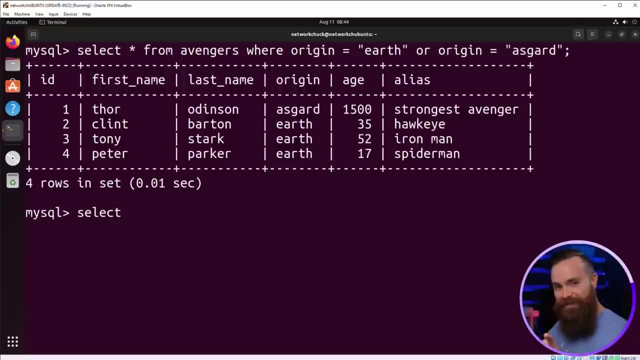 Let's try that, In fact, actually pause the video. See if you can do this. Pause, Unpause. We'll select the alias column from Avengers where age is less Than 30. We can do stuff like that, Bam. 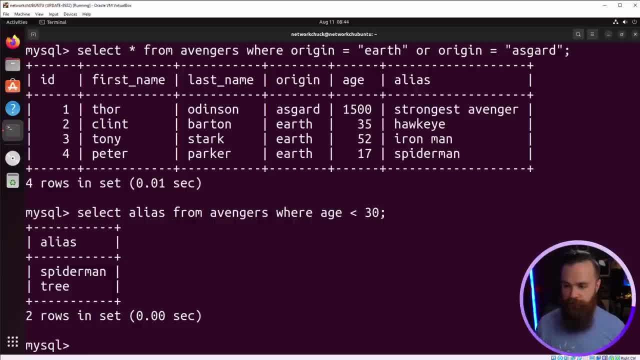 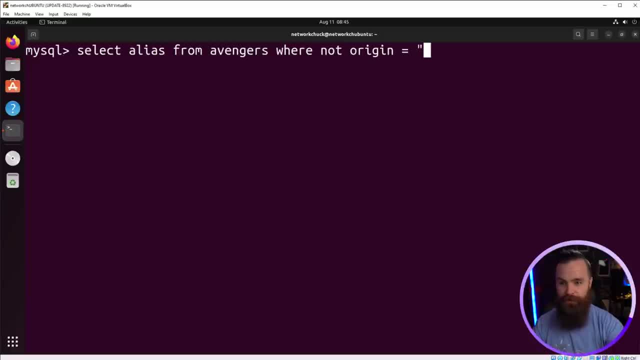 How cool is that? I just got the aliases Spider-Man and well Tree And there's pretty much an endless combination of how you can filter things. I can say where not origin equals Earth. I wanna see everyone that's not from Earth. 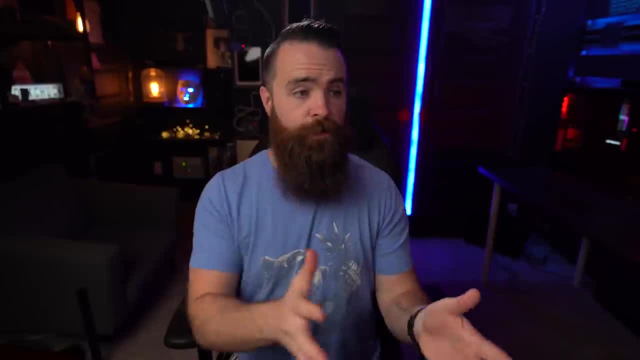 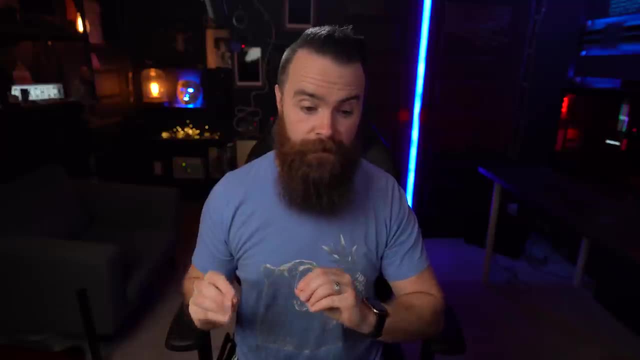 using our not statement. So you can go crazy with queries And often you may be typing in a terminal doing these queries- or it could be a GUI application or it's programmatic. You're programming things in Python to search for data with queries like this. 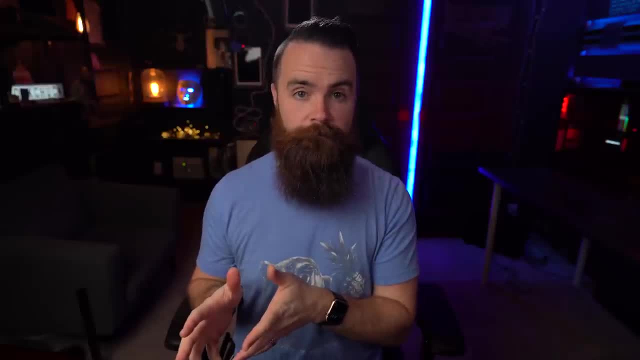 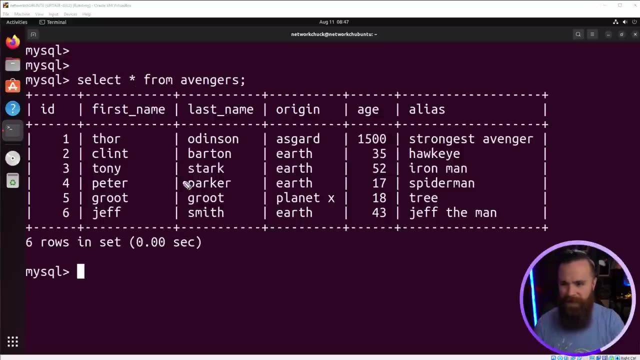 It's super powerful. Now, so far I've shown you how to add data to a table, but what if you wanna remove stuff? Cause did you notice this? Look at this. Some dude named Jeff snuck into my table. He's not an Avenger. 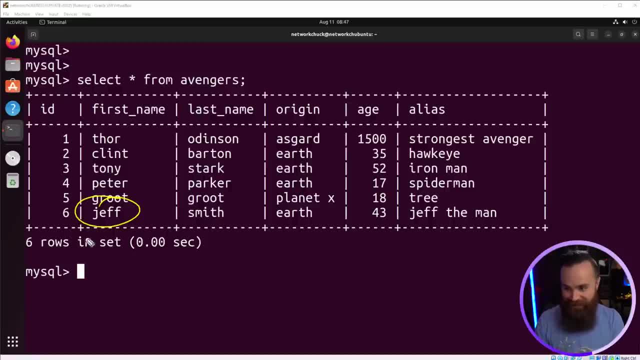 How'd he even get in there? So real quick, go ahead and add Jeff, add this data to your table and then let's remove him. So pause the video. real quick, add him and then let's remove him. We can remove the records from our tables. 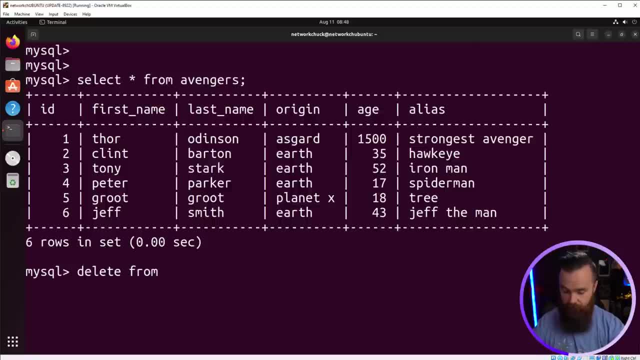 with the delete command We'll say delete. From then we'll specify our table Avengers and we'll tell them what we're wanting to delete. We could delete a lot of things all at once. gotta be careful, but all we care about is Jeff. 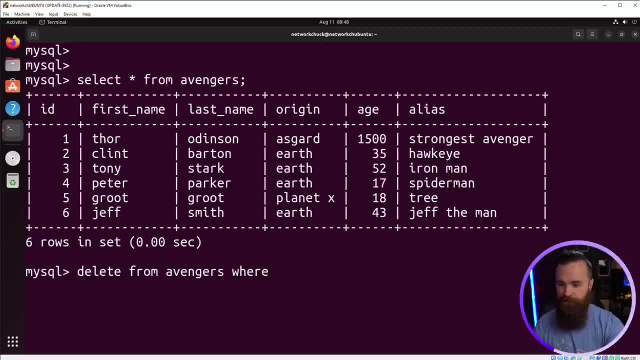 So we'll say where we'll use our filtering again, where we'll say: first name equals Jeff. That should do it. That should take out Jeff. Goodbye Jeff, And he's gone. I think Let's do our select statement once more. 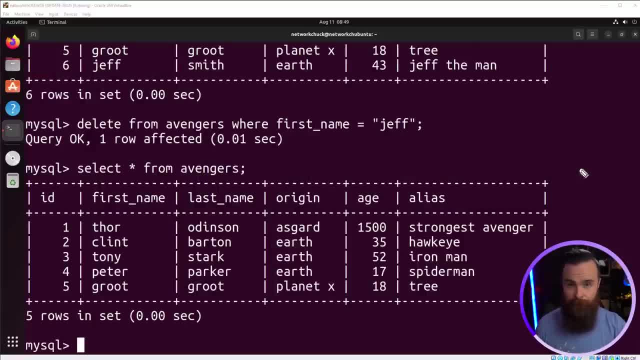 Woo, okay, Jeff is gone. Now we can also update the stuff in our table. For example, I was informed of this: Groot doesn't have a last name, It's just Groot, my bad, So let's change that. let's delete that. 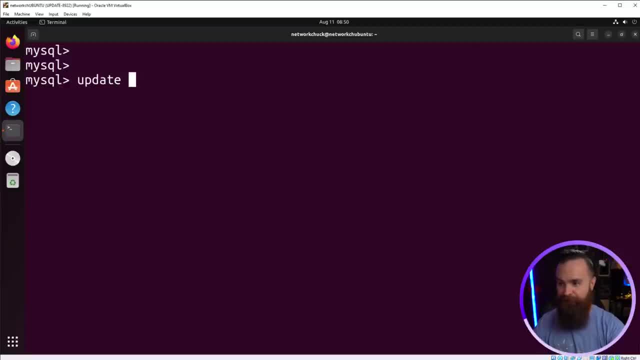 We can update entries in our table with the update command. We're gonna update Avengers and we'll use the set command to set a certain column equal to something. So we'll set last name equal to null, to nothing. That's how we do that empty. 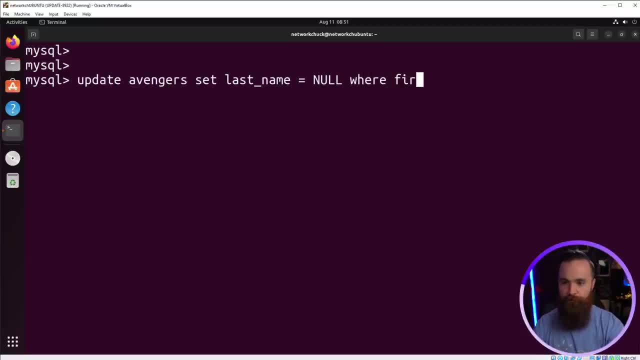 And because we don't wanna set every last name to null, we'll say: where first name equals Groot, That should do it. Let's try it out. Awesome, Actually, I didn't test this before. I wanna make sure it works. 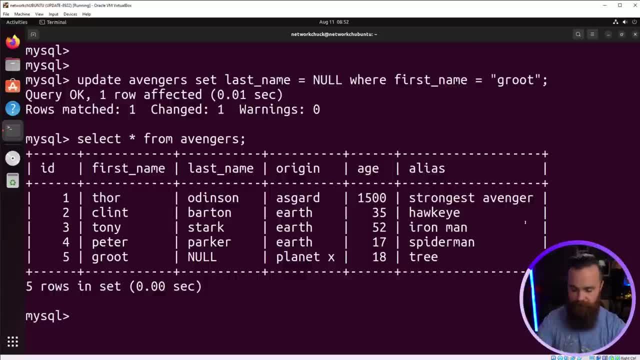 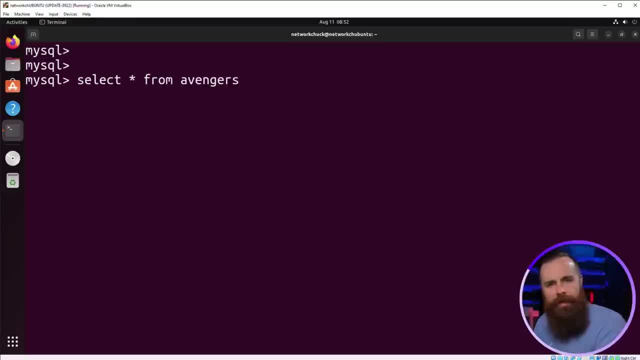 Excellent, Groot is now accurate and you guys can stop yelling at me Now. last thing on this: before we get kinda crazy, Let's go ahead and select all the Avengers once more, all their columns, But let's say we wanna see them in order of their age. 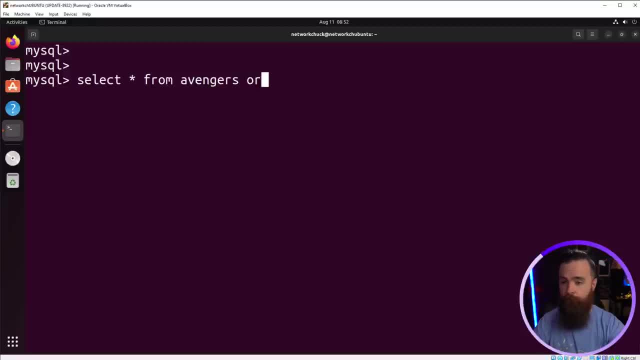 youngest to oldest. Let's see that We can do that by typing in order by the column age and we'll say: because we're going from younger to older, it'll be ascending, so we'll do A-S-C. Let's try it out. 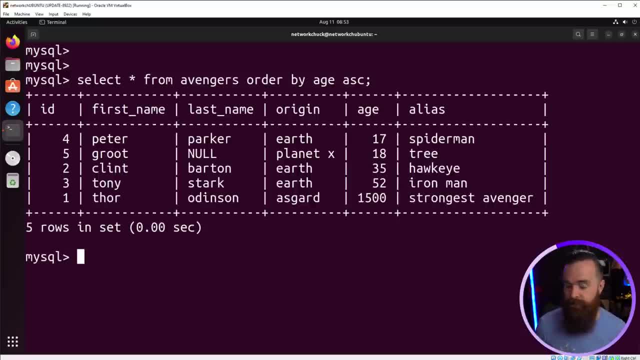 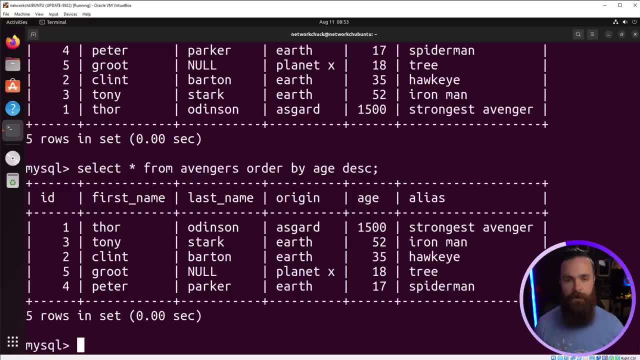 Perfect, look at that. 17,, 18,, 35,, 32,, 1,500, that's a big jump. Let's do it in reverse. Let's do oldest to youngest. We'll change that to D-S or sorry, D-E-S-C descending. 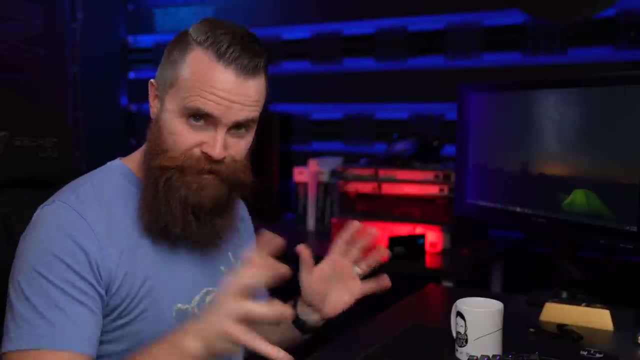 Awesome. Okay, last thing I'm gonna show you. maybe I might get too excited to show you something else, but we'll see. Okay, let's try this Right now. our table's looking pretty amazing. All the Avengers are here. 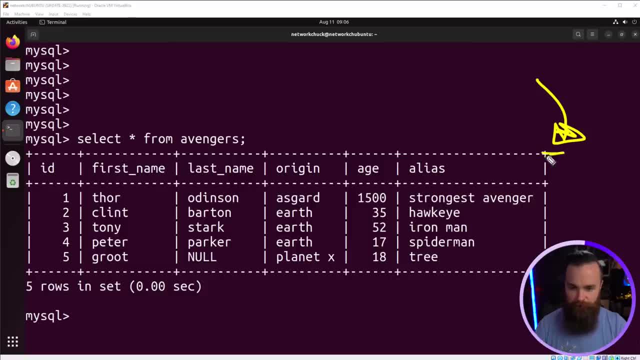 Well, some of them. But let's say we wanna know one more thing about them. I wanna know if they have a beard. So it'll be beard, and it'll be yes or no, or actually true or false. Let's do that. 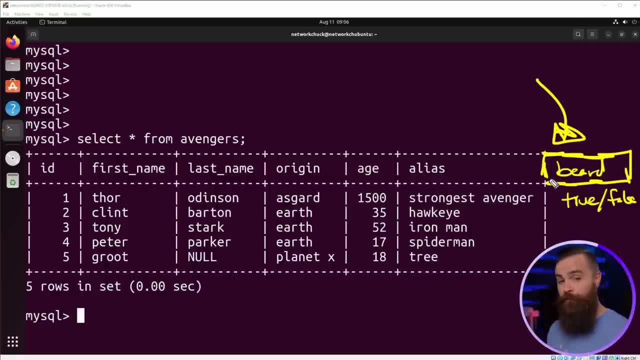 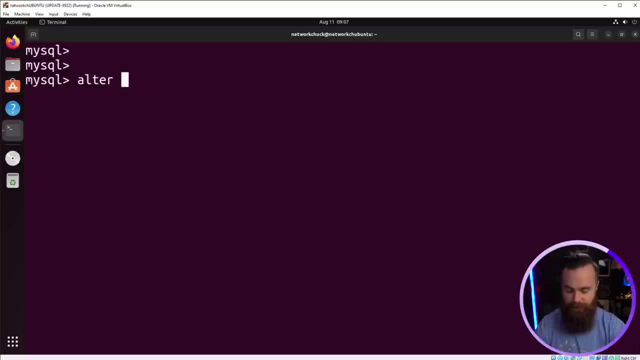 So here in our database, our table, we're gonna alter the table to have another column after it's already created. Let's do it right now. Pretty simple actually. The command is alter. We wanna alter it. We gotta tell SQL what we wanna alter. 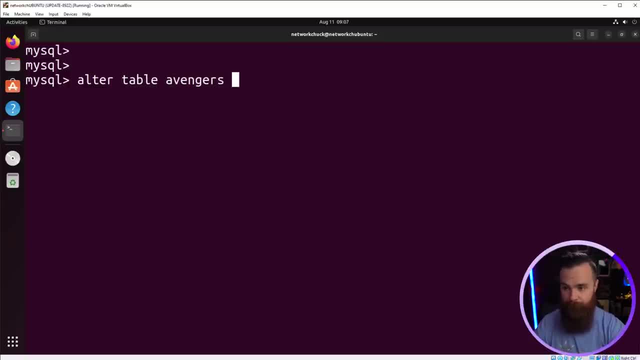 We're gonna alter a table, specifically the Avengers table. We're going to add a new column. We'll name it beard and then we'll tell it what type of data it's going to be. Now, because I want it to be true-false. 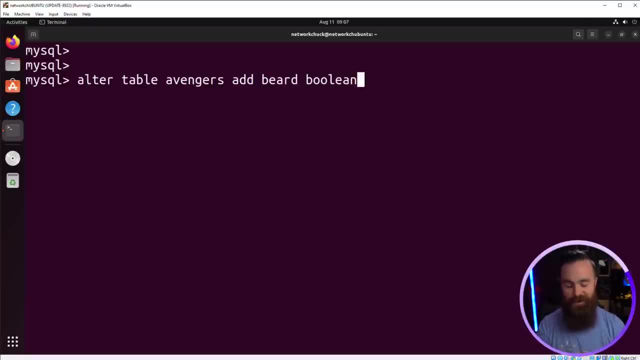 I'm gonna type in boolean, because boolean is true or false. That's a special data type. So here we're telling SQL, we wanna alter the table Avengers, and the way we're altering it is by adding the column beard with the boolean data type. 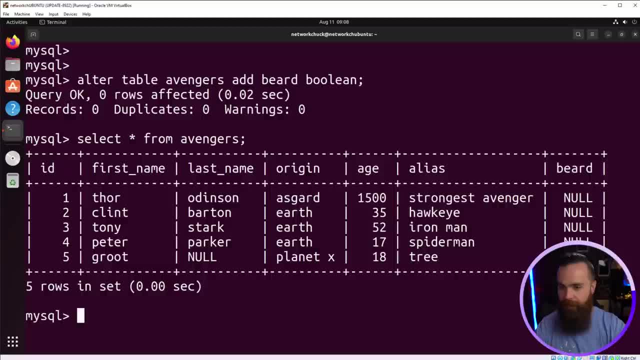 Hit enter, done. Now let's select and see what it looks like right now. Oh, look at that. New information, new column. Now here's a challenge for you. I want you to go in and update the record for the beard column for each of these Avengers. 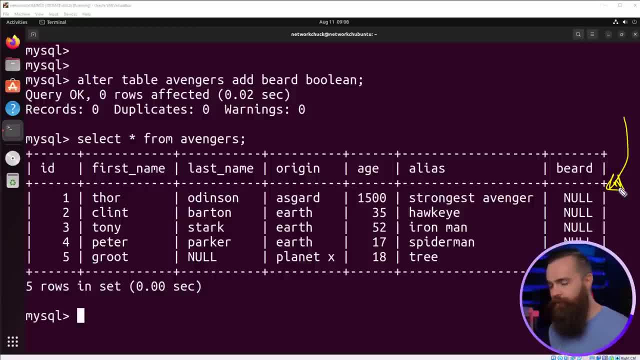 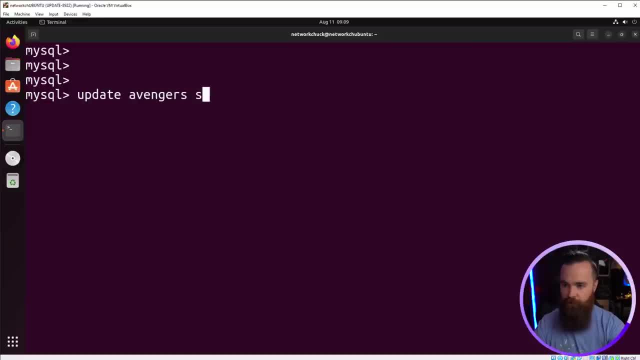 whether or not they have a beard. You should know that already, right? So go ahead and do it real quick. Pause the video Unpause. Here's how you would do that. like we just covered With the update command, go to the table Avengers. 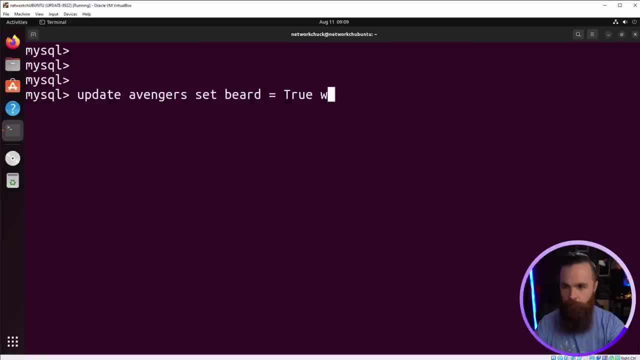 We'll set beard equal to true, where let's just say first name equals Thor, because we know Thor has a beard. Bam, let's see what happens. Perfect, and for Groot he doesn't have a beard, So we'll set beard to false. 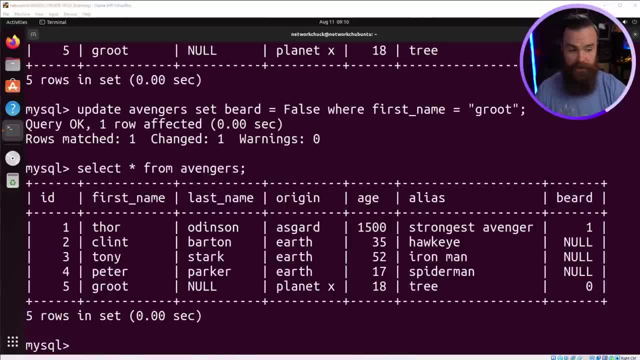 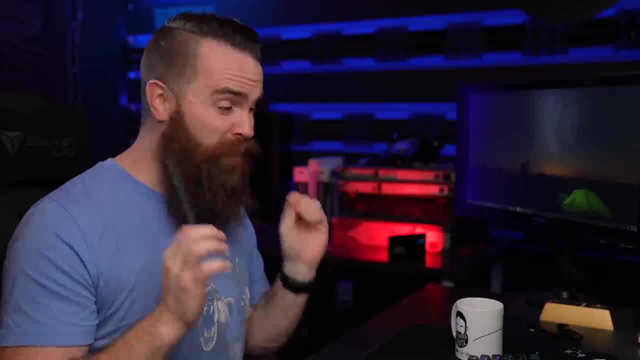 where first name equals Groot. Let's see what happened, Noticing that one is true, zero is false. Okay, we're gonna stop here. I could keep going. There are things I have not covered, but I don't wanna make this video too long. 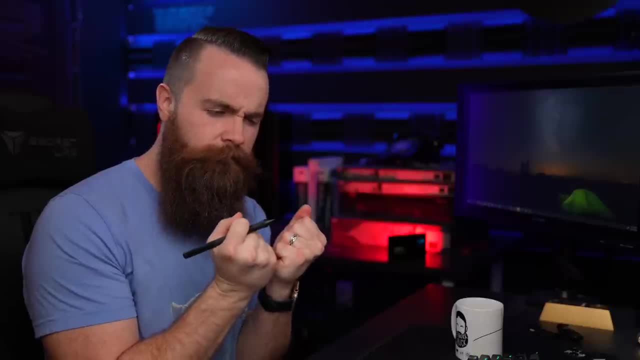 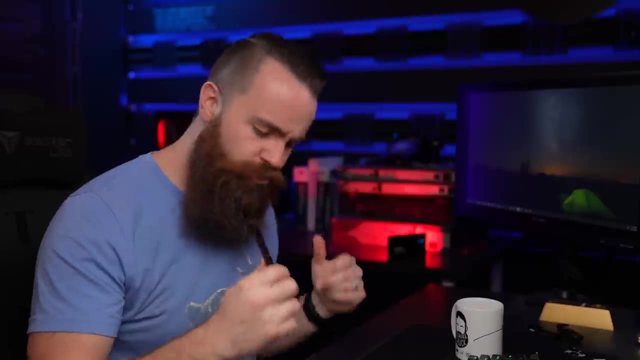 But I hope in this video I gave you enough to make you, like, feel semi-confident, Like I know what a database is, I can create one, I can select things, but also I wanna give you that hunger, that drive to learn just a bit more. 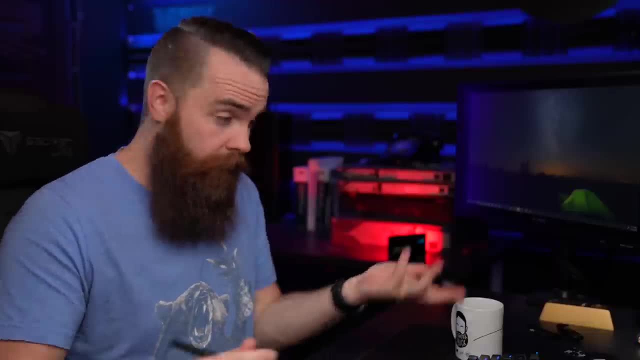 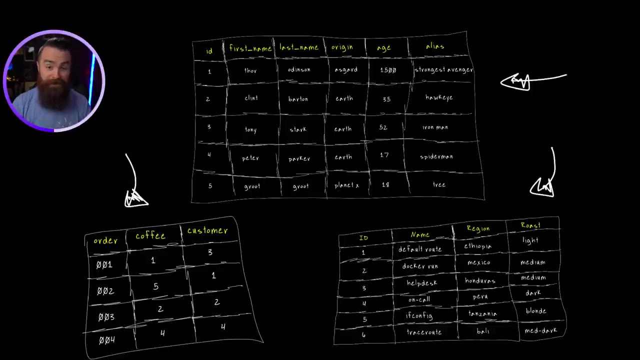 go beyond what I'm showing you here, Because there are things I didn't cover like look here: We did build these two tables inside our database, but we never built the orders table And, more importantly, we never built the relationships between all these tables. 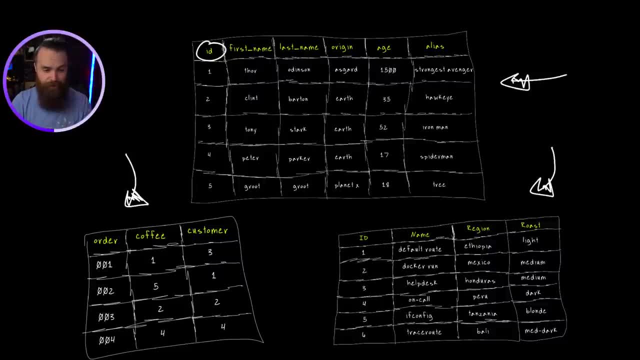 which would involve making the ID field of both our customers- our Avengers and our coffee- the primary key, And then when we reference those fields in our order table, those will be foreign keys And that unlocks the full power of relational databases. 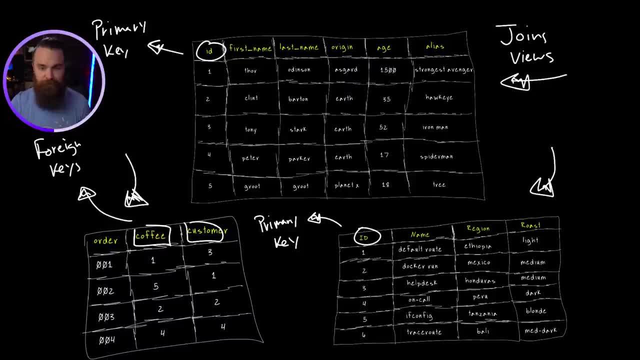 allowing us to do things like joins and creating views, which basically is pulling data from all these tables and only seeing what we want to see, Like: how many times does Spider-Man order the dark roast? We could find stuff like that, So I'm not gonna cover that here. 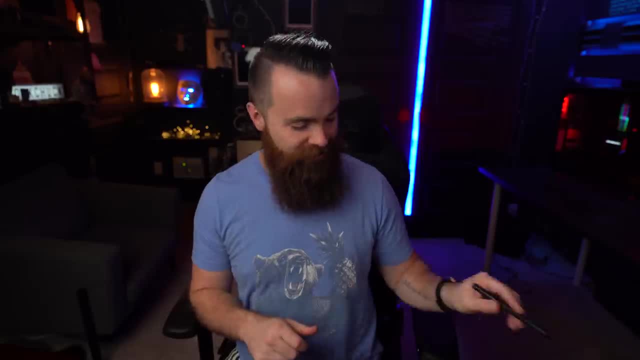 If you want me to create a video on that, let me know below. But anyways, that's all I got for today. Thank you for taking some time to have some coffee with me and talk about SQL Or S-Q-L. 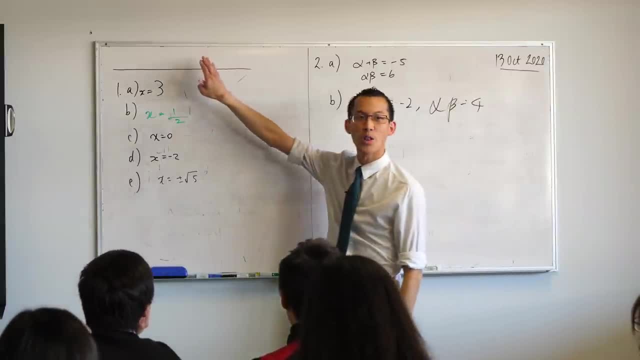 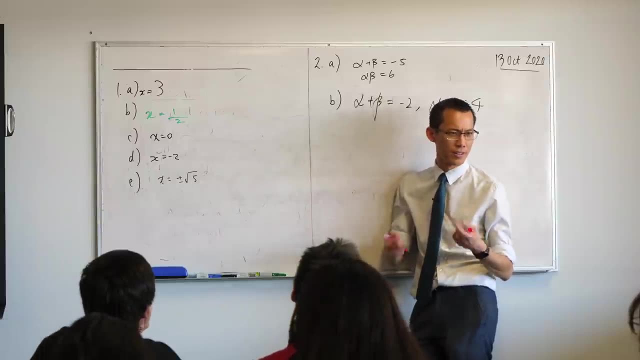 You'll find I often do this, but today what I'd like to do is leave space for a heading. I really hate when a heading is a spoiler for what you're actually going to learn. Don't worry, I'll fill it in, and if I forget, just tell me and then we'll fill it in. You might feel like these questions.